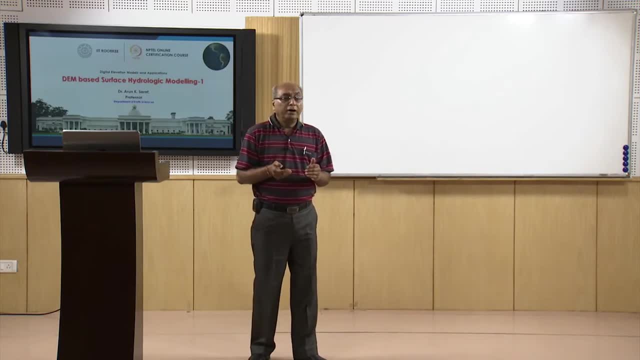 And also it is important to know that how these things are changing composition of area and how it affects the flow of water and what happens, because we want to simulate the conditions- and that what happens when deforestation occurs, or what happens when deforestation is done to the water flow or to the soil moisture conditions. 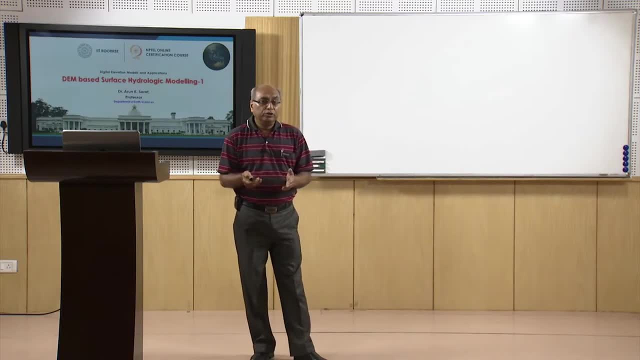 So these things can also be modelled using our surface hydrologic modeling models and based on DEMs, and how this can affect at a watershed level, catchment level or a basin level. that can be because these are the hydrological boundaries- the watershed, catchment or basin- and therefore 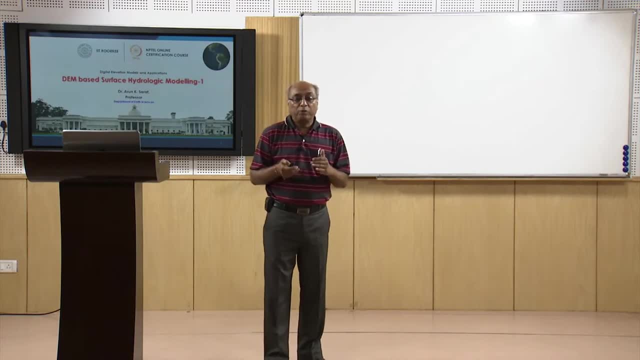 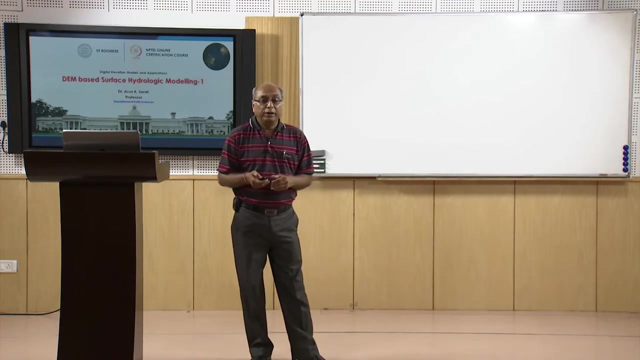 generally when, whenever we work for a problem which is related with hydrology, Then we have to look for natural boundary rather than political boundaries, and also how we can mitigate a problem. may be a soil erosion problem, may be a flood problem or so on, So these can also be there. also, we can use these approaches, that is, surface hydrologic modeling. 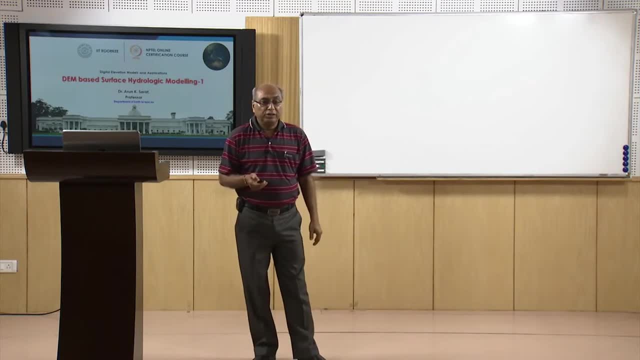 There are various applications, some of which we will be seeing in this discussion. So first, before we proceed for a typical surface hydrologic modelling steps, which is a sequential processing, We would like to understand first what is basically drainage system is. So this is the area upon which water falls, like a watershed, boundary, and the network. 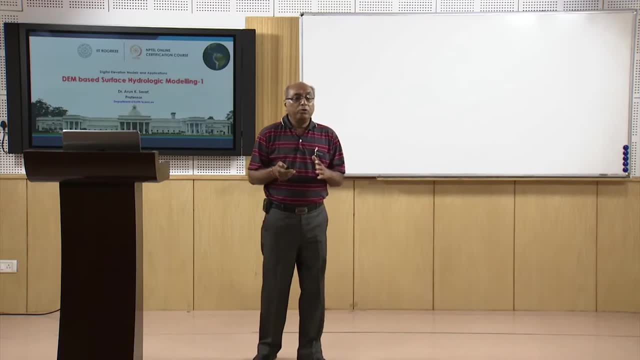 through which it will travel to an outlet is referred as a drainage system. So there is a network of drain lines starting from 1st order stream to 2nd order, 3rd order, depending on the size of the basin or watershed and the water which will come as input. as 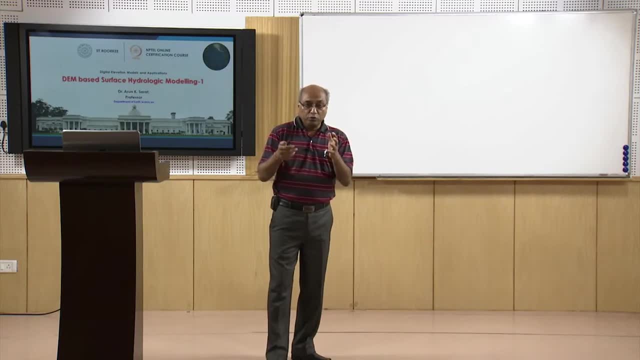 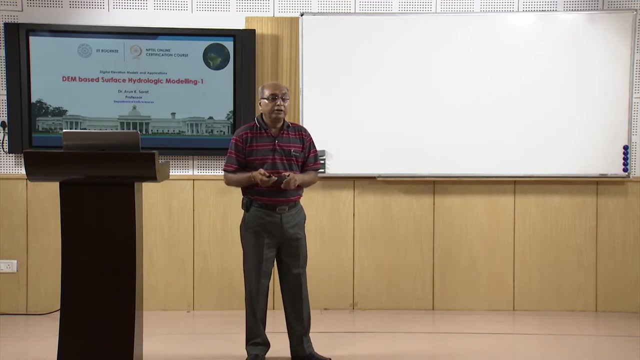 a form of rainfall or precipitation has to flow through this network. So where it will flow, exactly how it will follow, this will depend on elevations, and that is why elevation models are used Along for in the in surface hydrologic modelling, to drive drainage network as well and the flow. 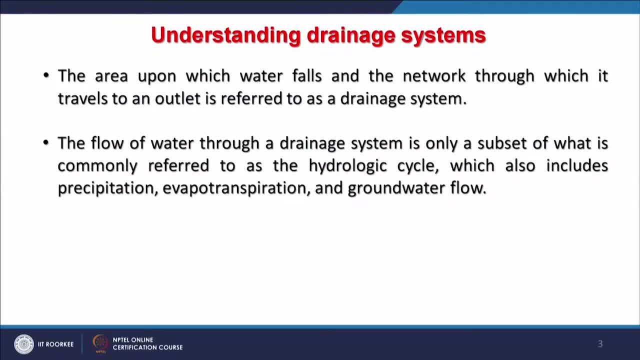 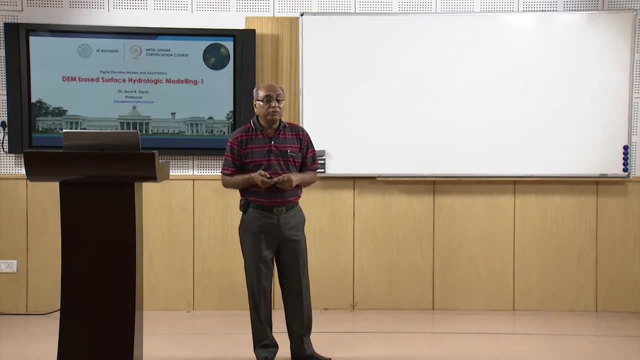 of water through a drainage system is only a subset of what is commonly referred to as a hydrologic cycle and because it is a it is a hydrologic cycle encompasses the complete flow of water, or movement of water through all processes, But it this drainage system. 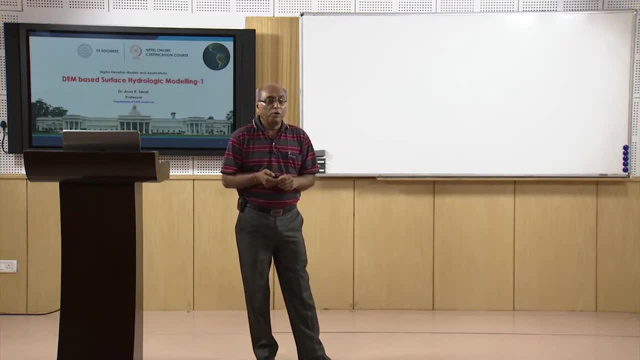 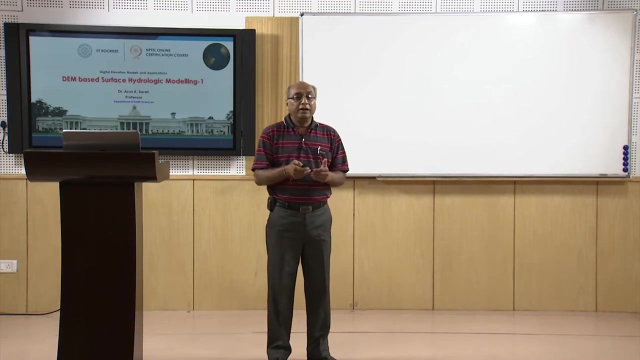 The flow of water in a drainage system is just a small part and which, but which is the hydrologic cycle, includes precipitation, evapotranspiration and groundwater flow, whereas in directly in surface hydrologic modelling we cannot handle like evapotranspiration issues or outputs. 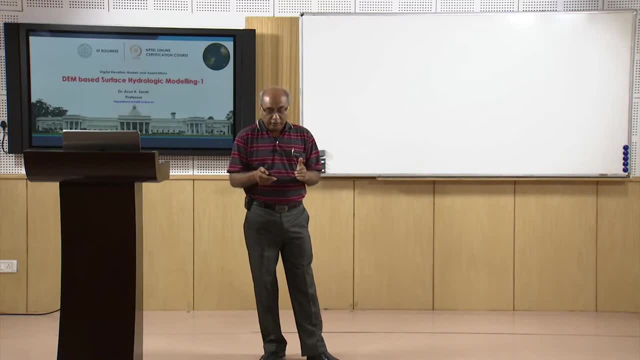 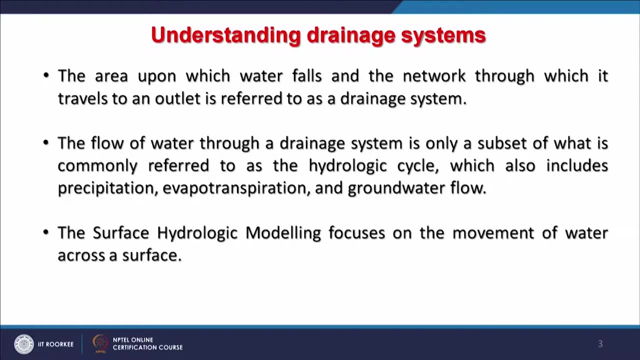 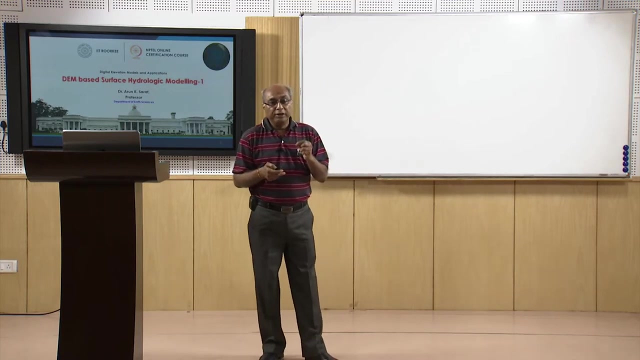 or in or groundwater flow as well. So, but overall, this hydrologic cycle, Hydrologic cycle will include all these Surface hydrologic modelling. that is why name says it only take care about the water which is flowing on the surface of a terrain, on an area, and assumed assumption is that every 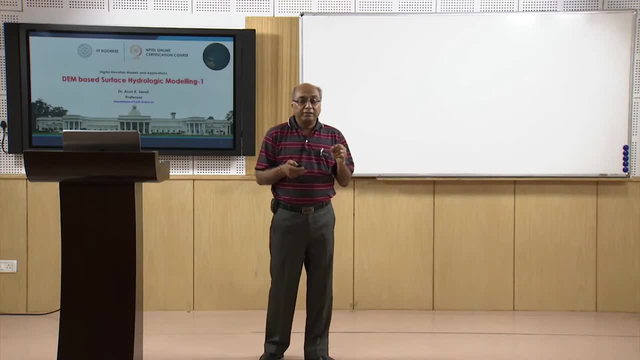 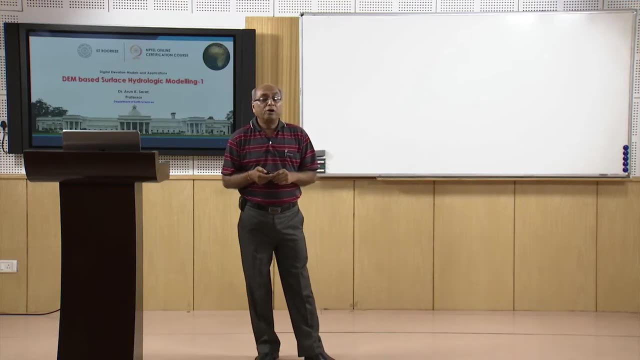 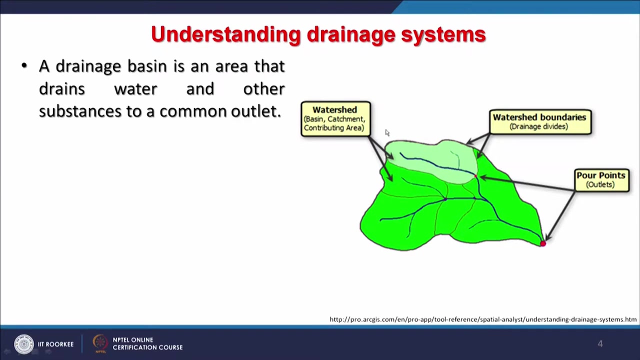 drop of water will flow over that as a surface runoff, So this has to be remembered here. So surface modelling focuses basically on the movement of water across a surface, Over land flow or surface runoff, which we talked. So here we are having a drainage basin or a one large one. is there a watershed boundary? 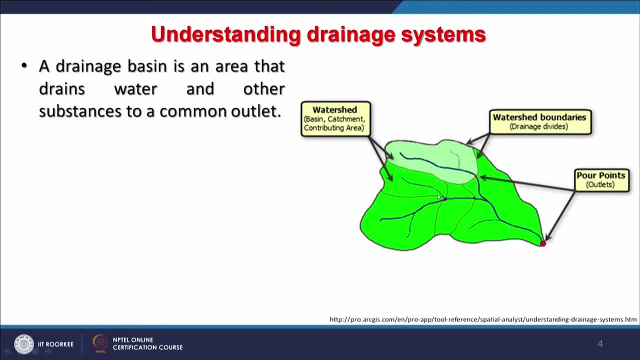 is also there and in this schematic We are also having a drainage network and this is the outlet, or also called pore point. So for a larger basin, the pore point is going to be here. for a smaller watershed or a sub-basin, So for a larger basin, the pore point is going to be here. 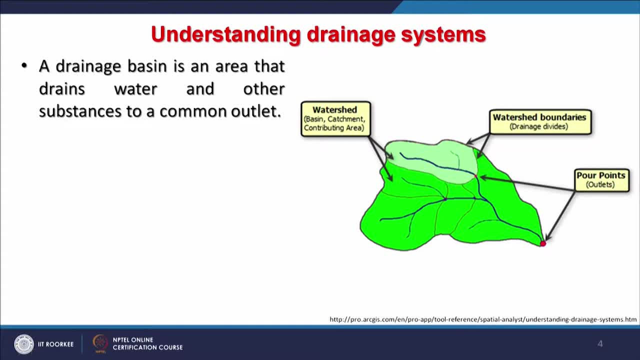 For a smaller watershed elevation, it may poor point may be in the upstream area, and this is. these are the boundaries which we call as hydrological boundary rather than political boundary. These hydrological boundaries are based on elevations and this is what the surface hydrologic 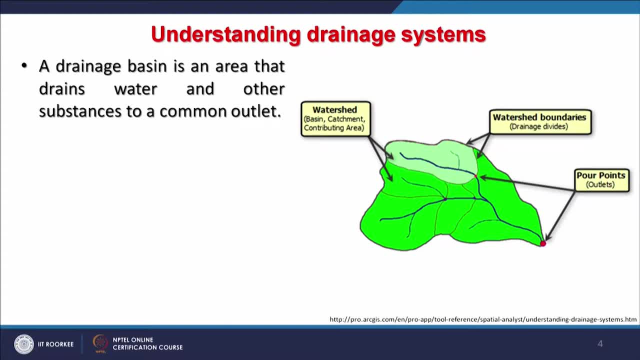 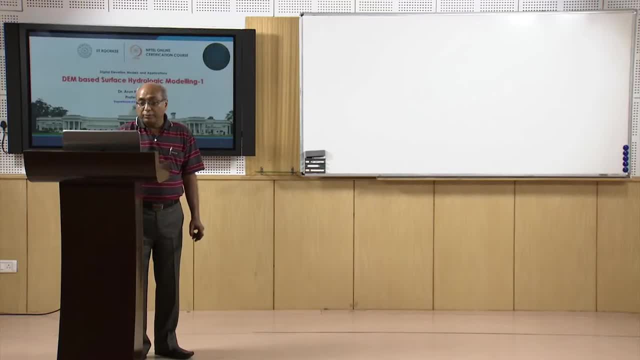 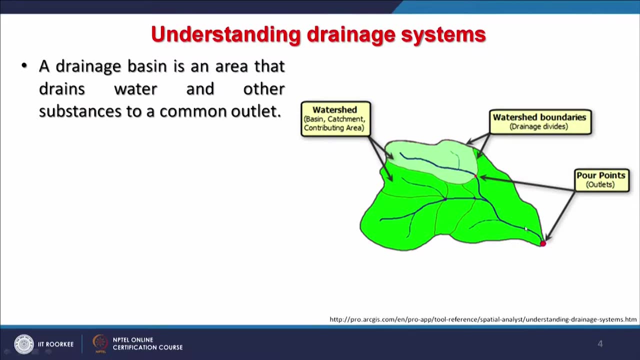 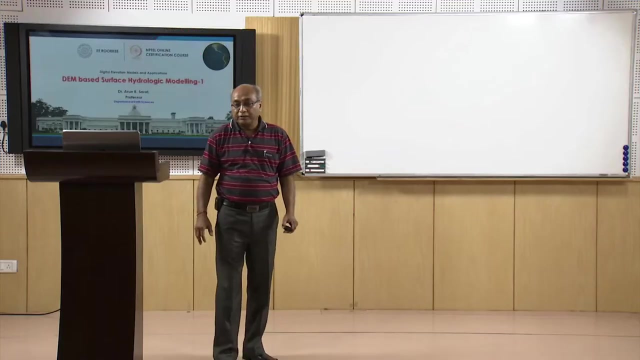 modeling exploits, basically because water will also flow through low elevation areas surrounding. may be you may be having higher areas, but water will flow through the always the low elevation areas and to further low elevation areas and therefore it will create a track and this is that we call as a drainage network. 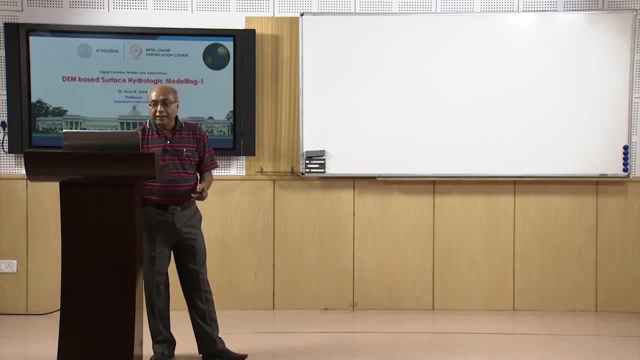 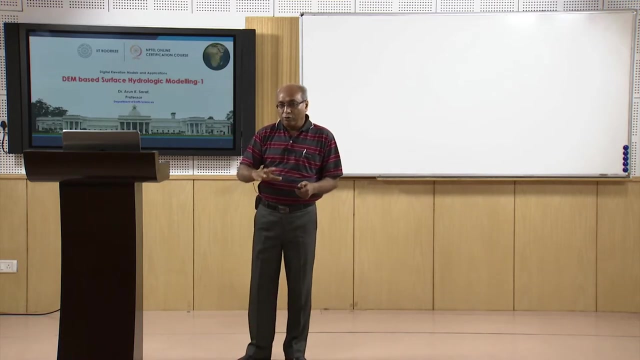 So the drainage basin is an area that drains water and other substances to a common outlet. These substances may be Sediments, may be nowadays pollutants, or other things as well. So whatever is will flow through this drainage basin at that particular outlet where we are. 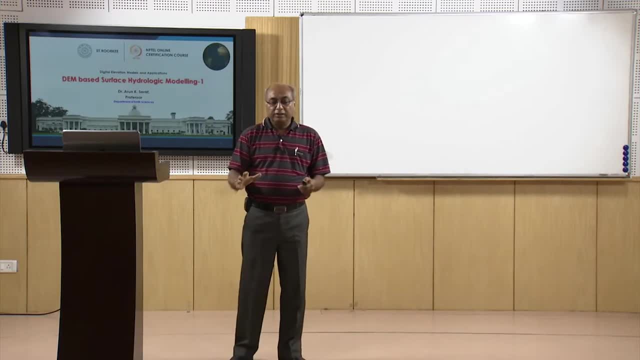 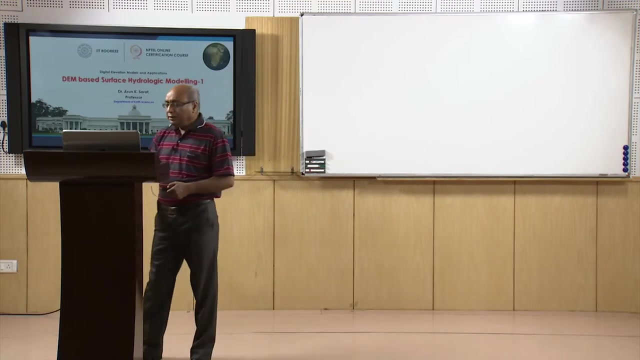 deciding that this is going to be our outlet. In this surface hydrologic modeling, a user can choose interactively where he is going to choose the outlet and, accordingly, a watershed boundary will be drained. There are other terms which are used for drainage basins. 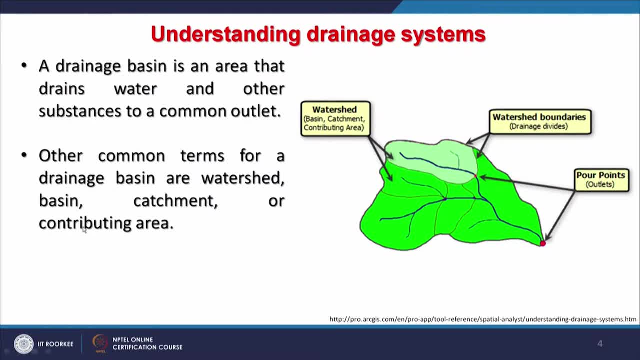 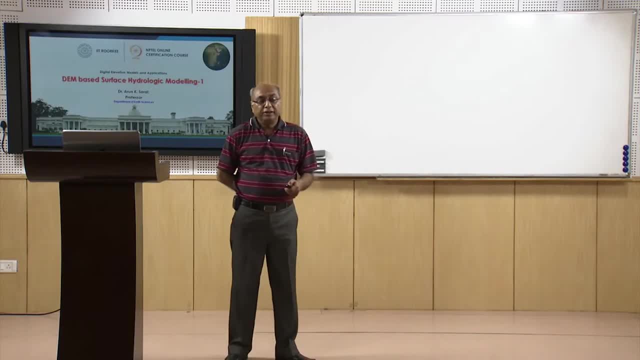 For example, unlike watershed basin, a catchment or a contributing area, and a opposite to this is a distributing areas which in civil engineering or in hydrology it is called command area for a canal network or some other thing. So that is just opposite to our drainage basin or watershed boundary or watershed basin. 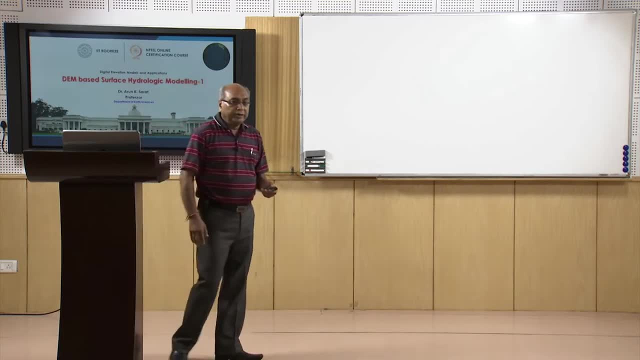 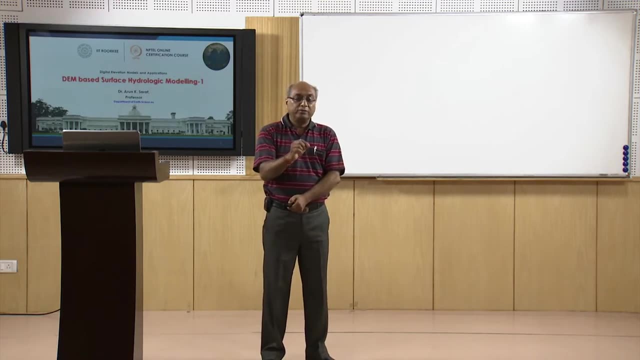 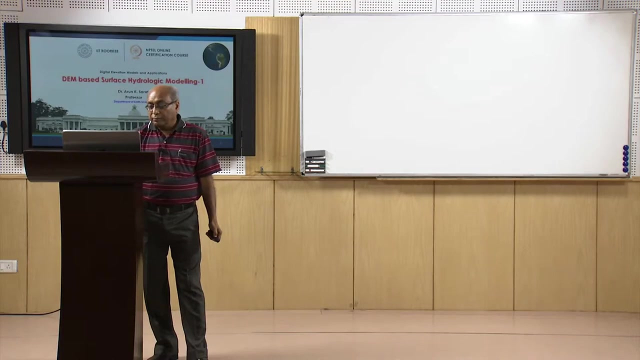 And In this area is basically normally defined as the total area flow to a given outlet of a pore point. So the outlet is very important, where we are choosing the outlet. if we shift the outlet at, say, this location, then we may have a watershed of this much size. but if we go downstream, 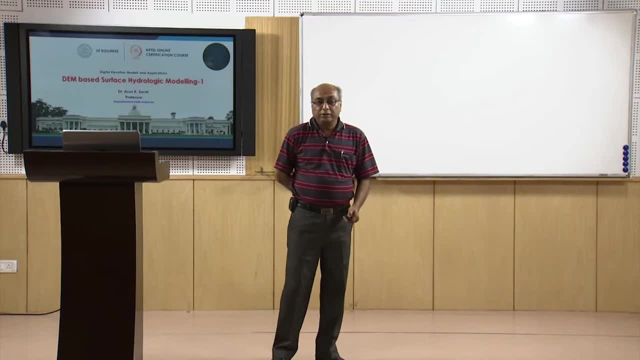 for the choosing the outlet. our basin or watershed will become larger and larger, So this has to remember the pore point. The pore point is the point at which water flows out of a watershed. So again, as we have discussed that pore point, from where the water will come, or whatever, 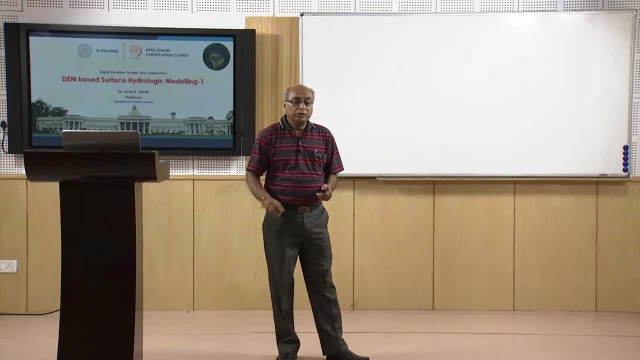 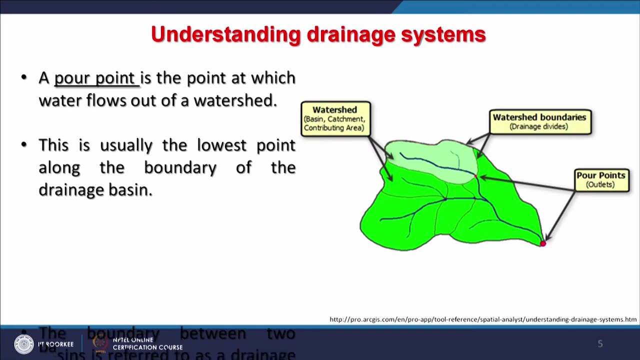 the sediments and other things will come, And this is usually the lowest elevation point of a along the boundary of a drainage basin. Note may not be exactly within lowest point within the watershed, but at the boundary of a drainage basin or watershed boundary and between 2 boundaries of our between boundaries. 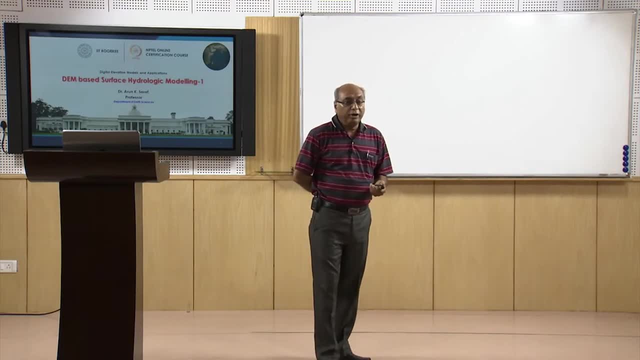 of 2 basins. it is referred as watershed divide or watershed boundary as well. So because topographically it makes a basically a ridge and that ridge will not allow water, will allow water to flow either in one basin or one watershed or another one. 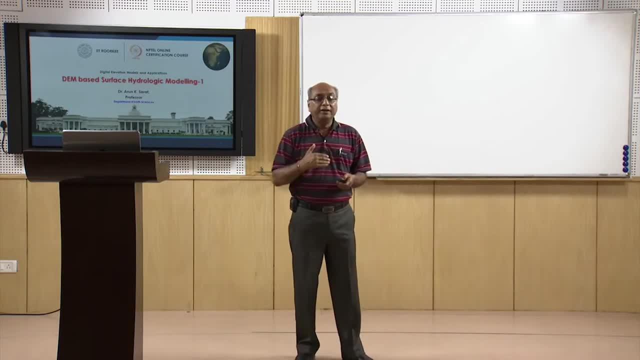 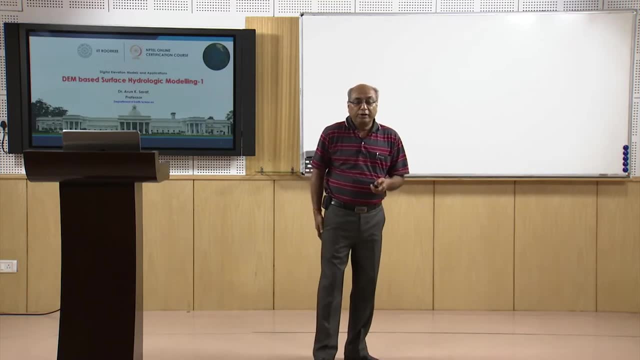 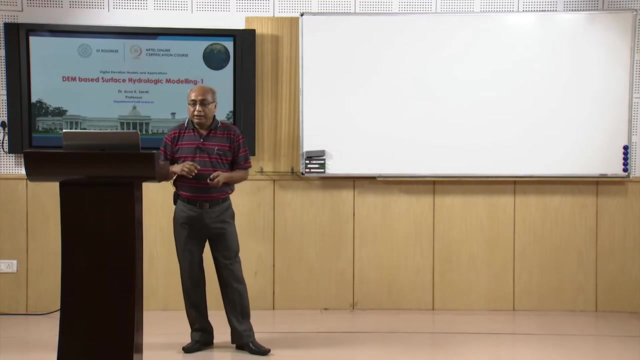 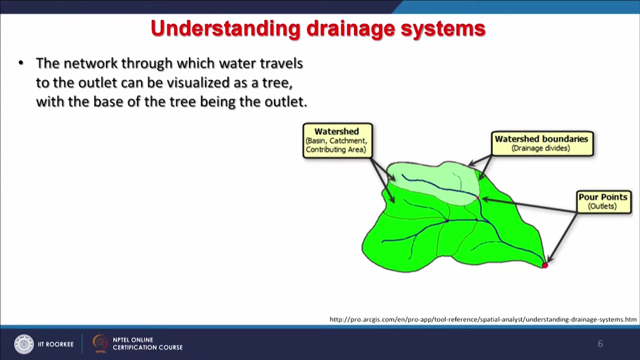 So that that that ridge, That ridge serves as a divide and therefore sometime people call as drainage divide, or that also becomes watershed boundary or basin boundary. Now the network through which the water will travel to the outlet, which is in this schematic- it is shown as a red points- as either is large one or a smaller one, and this network can. 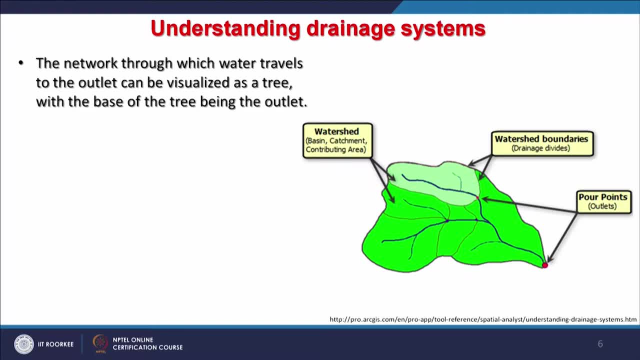 be visualized as a tree, with the base at the tree being at the outlet, And there are, though patterns are there, but we will discuss a little later- and branches of these trees are a. basically, these are the stream channels, or these are the drainage lines are there and the intersection of 2 stream channels is a referred to as a node. 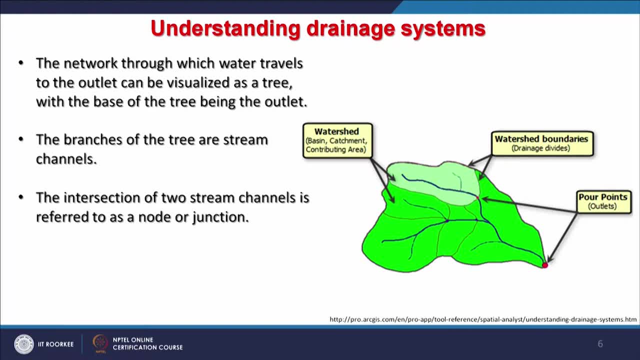 or junction. So if we, So if we, If we talk in terms of vector data and the same concept is used when 2 vector lines meets, then we say node or maybe inter node and other terms can be used similarly here- that intersection. 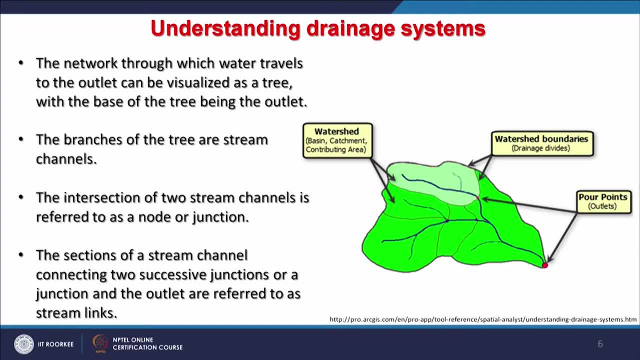 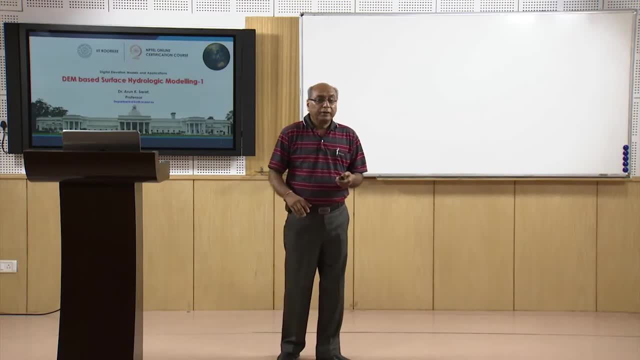 of 2 stream channels is referred as a node, and the sections of a stream channel connecting 2 successive junctions or a junction and the outlet are referred as the stream links. So these are important While doing, While doing surface hydrologic modeling. 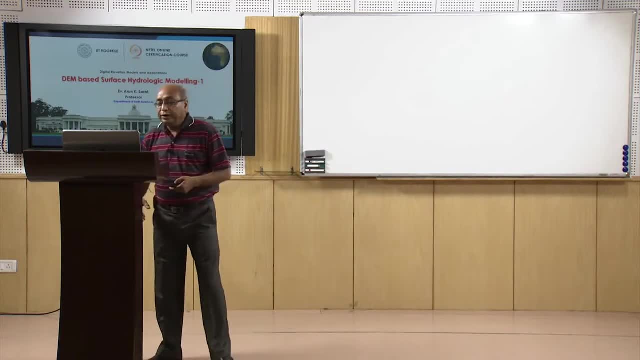 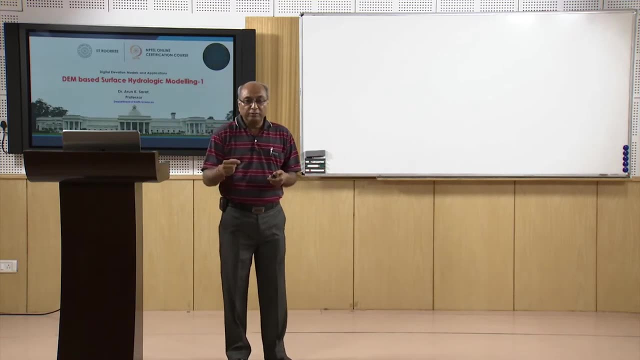 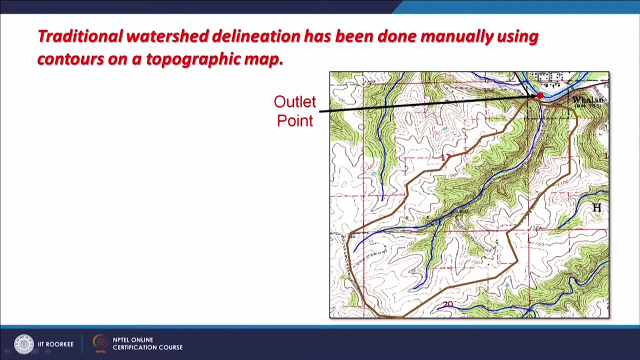 Now here, traditionally what we have been doing in order to drive the watershed boundary, we used to have a topographic maps and in which, based on the contours, we used to drive or delineate a watershed boundary. and this is once we decide the outlet. suppose outlet is. 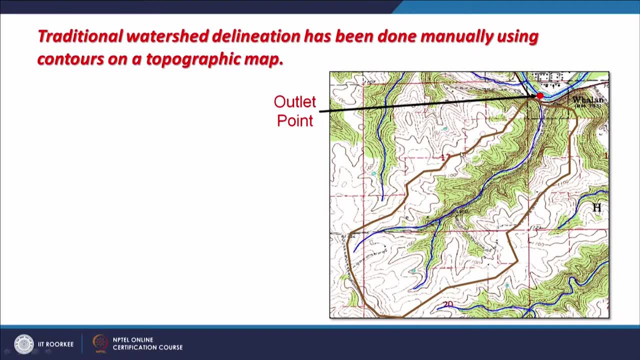 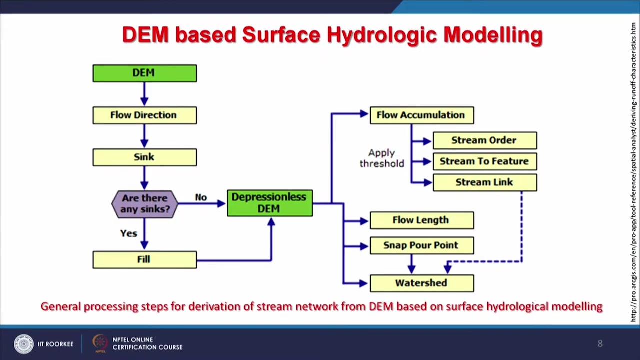 decided at this location, then delineation will start following the contours which are making the ridge, And likewise a watershed boundary can be delineated. So traditionally, this is how manually this was being done- that we sketch throughout this thing: following the watershed boundary, But in a in a, on a GIS platform, using a digital elevation model and employing surface hydrologic. 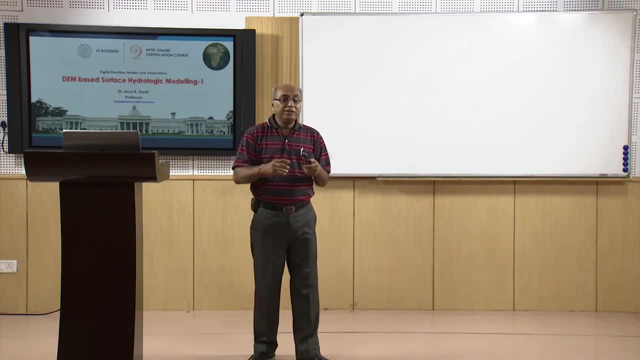 modeling. We can delineate watershed boundary At At At At any location within our digital elevation model and it is after certain steps of processing. it can automatically be delineated if we decide the size of basin. So if we say that I am, I want to delineate all water sets which are having 500 area equal. 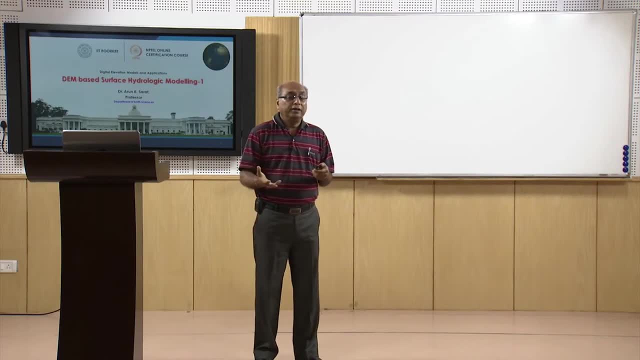 to 500 square kilometer or more. Then say: then through surface hydrologic modeling, This can be done automatically for a a large area, whereas in manual method, for individual watershed boundaries have to be delineated. Now we will go through one by one about this surface hydrologic modeling processes, which 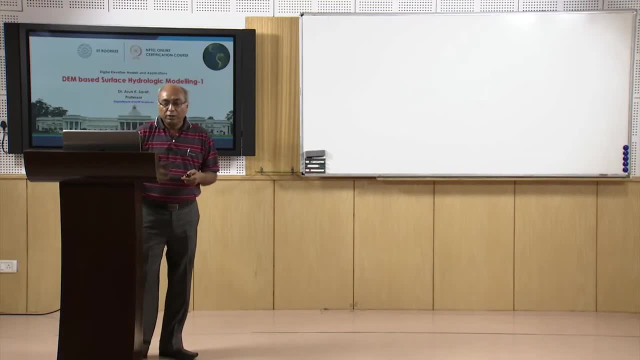 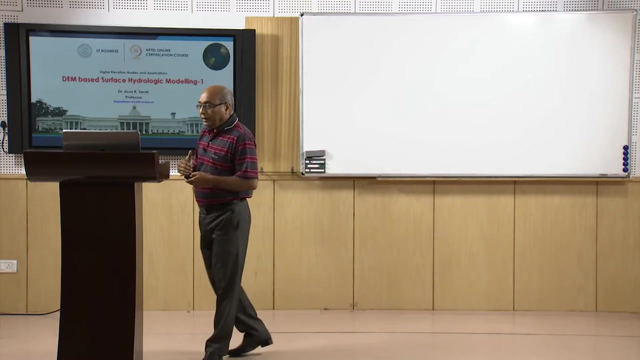 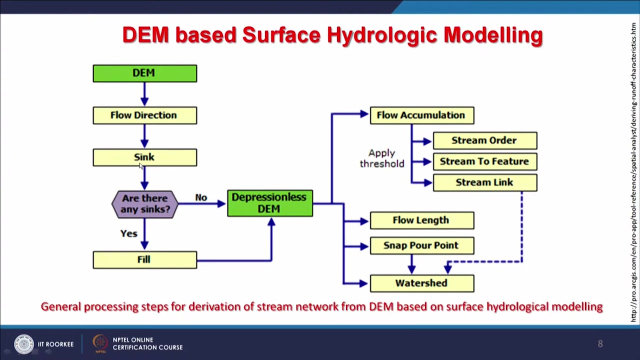 are there, as I have mentioned, is a most of most of the process are in a sequence, So we will go one by one. Like First What we do. We take a digital elevation model and drive directly flow direction And, again using the same digital elevation model, we can, we can drive a, find out where. 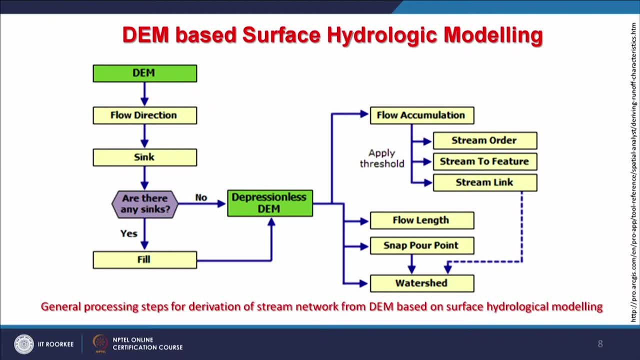 are the sinks or artifacts in a digital elevation model, because digital elevation models may have some errors and why these sinks are identified. or depressions, local depressions of one pixel, one cell size Or maybe two cell size and sinks are. or depressions are identified because water has to flow on. 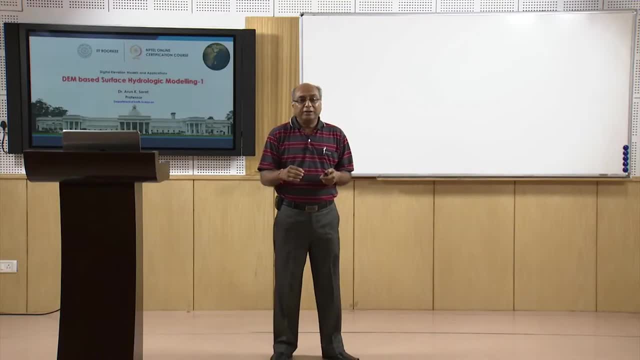 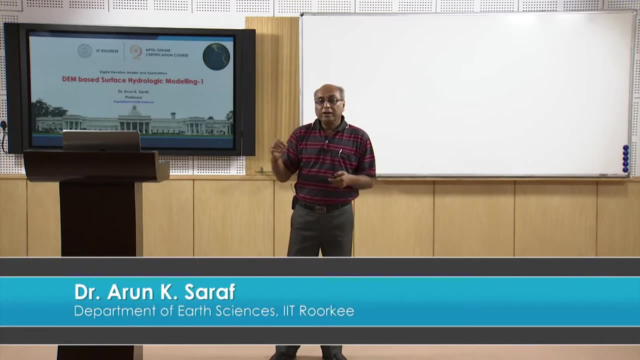 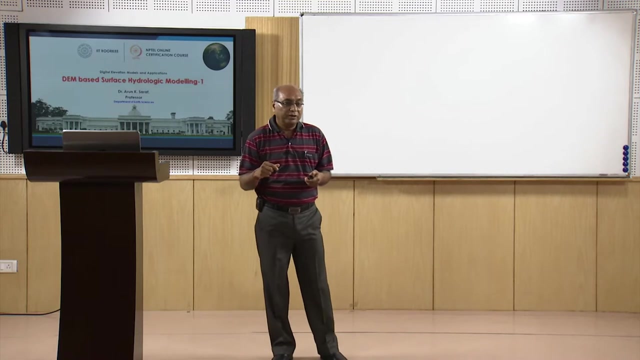 the surface. It cannot remain intact or remain on one place, because this is what in surface hydrologic modeling is say, it is delineating or it is basically assuming that water has to flow on the surface as surface runoff and therefore these sinks have to be identified and later, 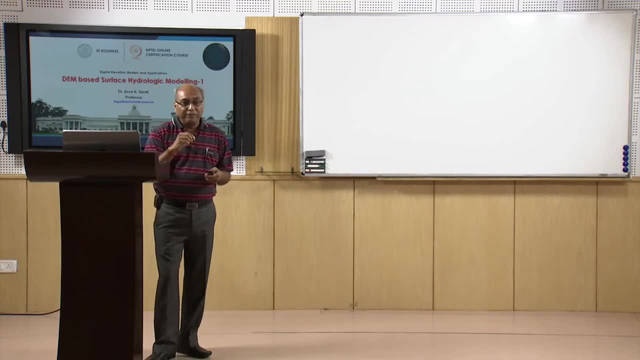 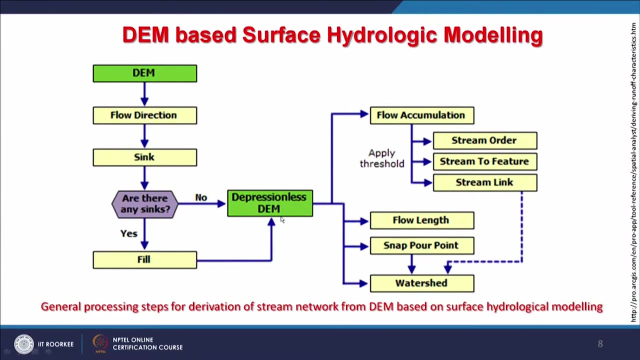 these sinks. if they are there, these have to be filled, and once you have filled, and then you are having a depression, less digital elevation model: One output: we have already created a flow direction, and then we are having a depression, less DEM. So these two outputs will allow us to create one more layer or theme, which is flow accumulation. 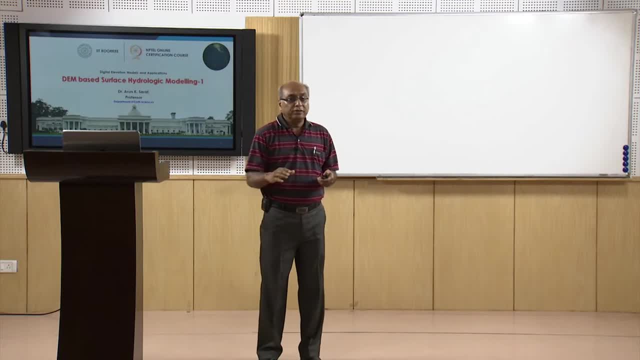 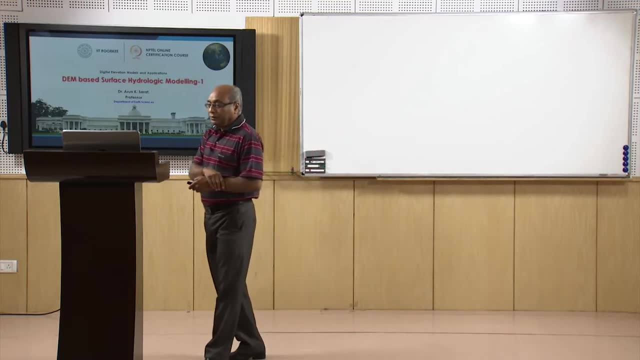 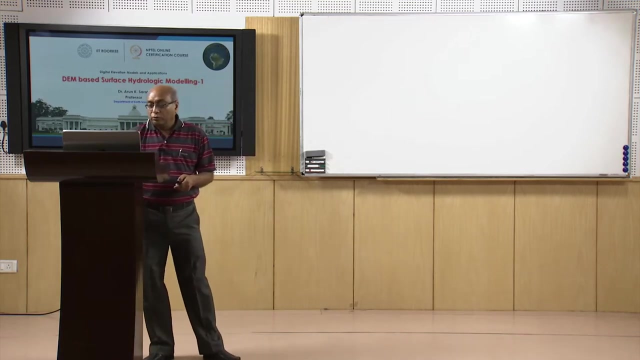 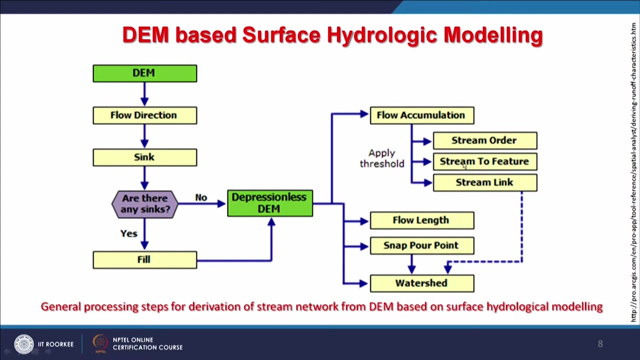 Okay, And once we reach to this stage, which is a very simple, very quickly one can perform and can reach to these three products, that is, flow direction, depression less DEM. This depression less DEM and flow direction goes to calculate the flow accumulation. This flow accumulation can be used to calculate stream order, stream and links and other things. 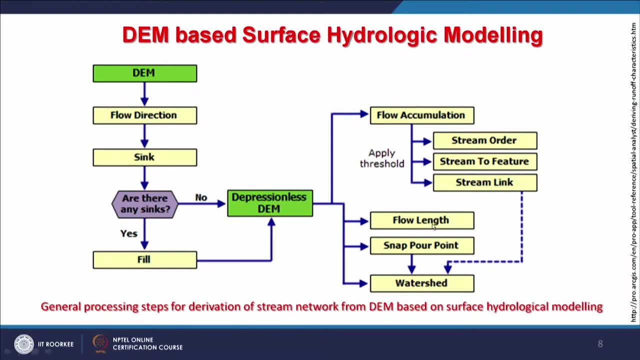 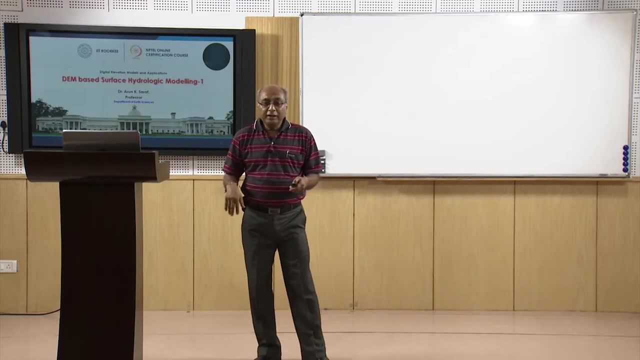 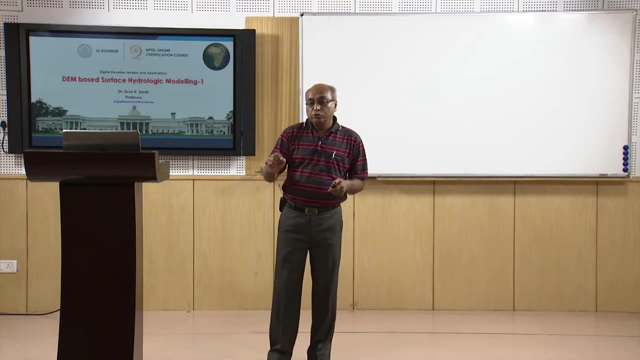 are there. It can also be used to calculate flow length. So that is why the flow chaos and depth ratio twice, this flow time once and then all values which are there in head is un AirPods. So this is what we are doing. 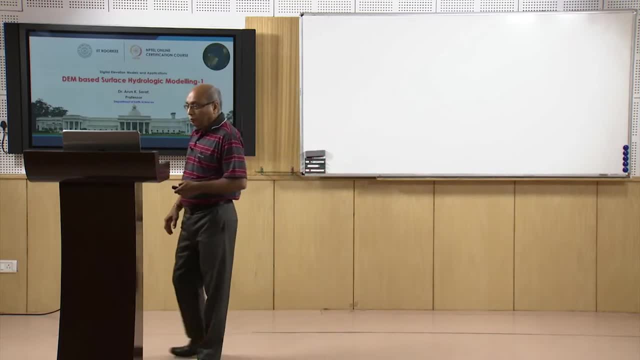 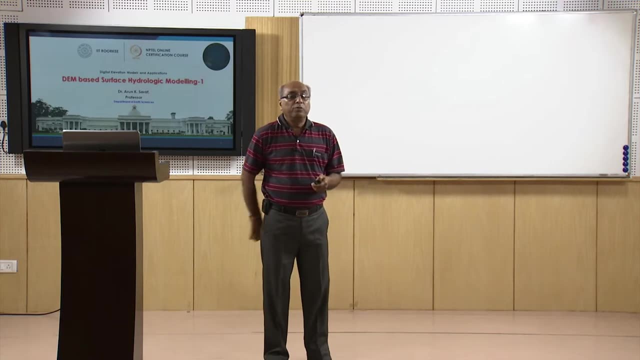 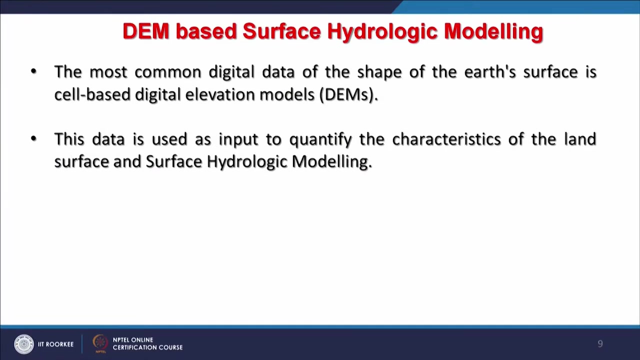 Okay, I will be showing through few slides And basically the most common digital data of the shape of the earth surface, as we know, is the DEMs, and these DEMs we used- and the data is this DEM- as an input, basically, which quantify the characteristics of the land surface and surface hydrologic modelling. 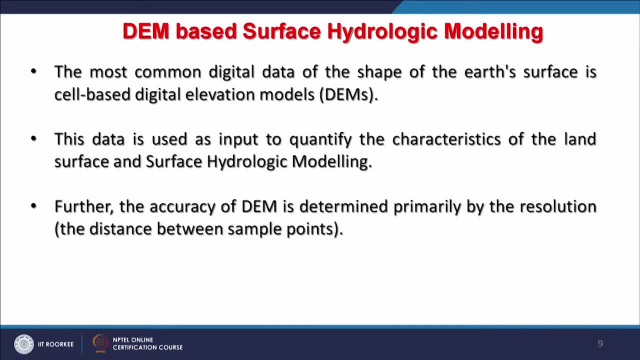 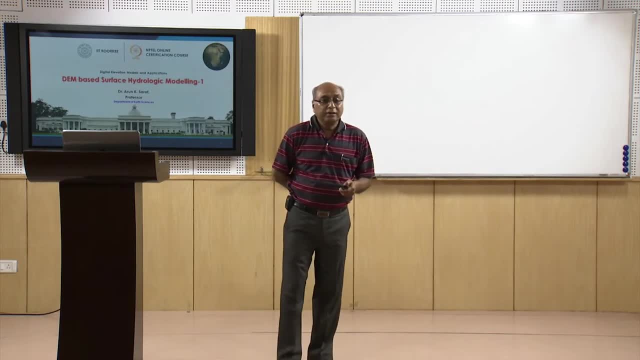 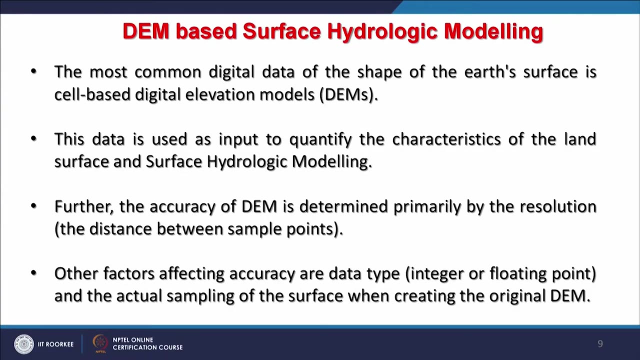 Further, the accuracy of DEM is determined primarily by the resolution. So always for this kind of processing, a better or higher spatial resolution DEM would give us the better results. and the factors which basically affect the accuracy are the data type, that is, the cell values of a digital elevation model, whether we are having in digital 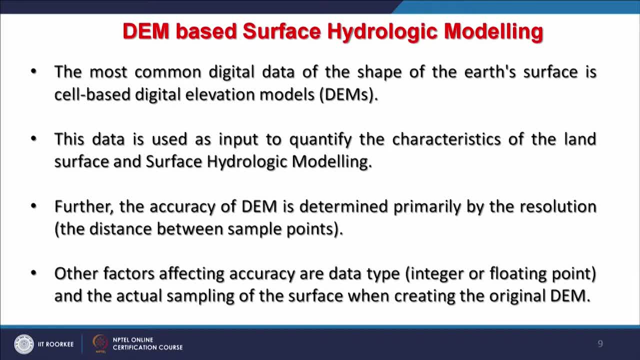 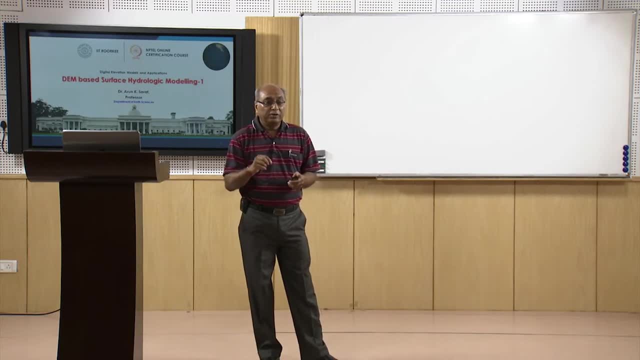 measure value or real or floating point value. they will influence sometimes our results, but generally in a digital elevation model we are having a real values or floating point values and actual sampling of surface where this surface hydrologic modelling will be performed. of a original digital elevation model. 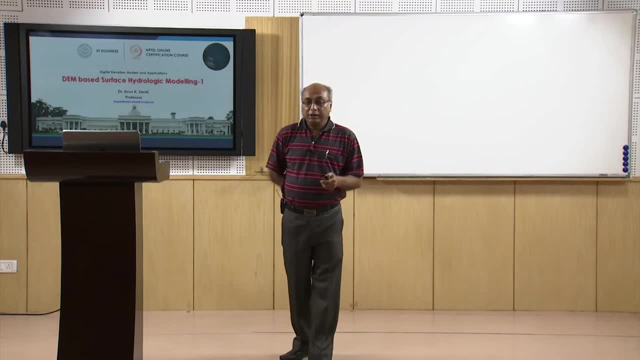 So these things will influence our surface hydrologic modelling outputs. Thank you, Thank you. As you know, the errors in DEMs are usually, as mentioned, can be classified as sinks, depressions or maybe peaks. but for a very small area, not very, maybe 1 cell size, 2 cell size, not more. 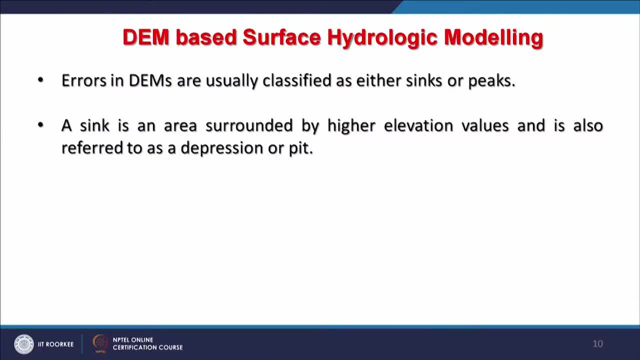 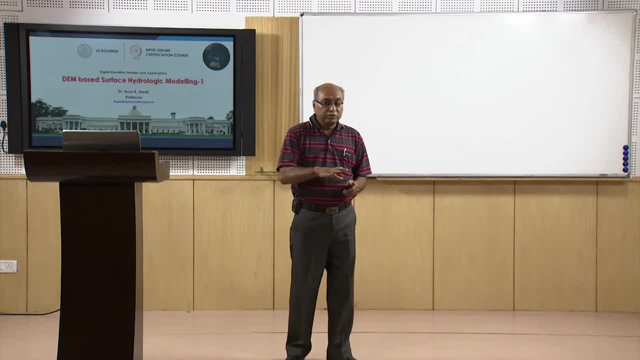 than that. So we consider them as sinks and we identify them in the very first few steps and then fill that, those sinks, using the surrounding values So that the water can flow. Water can flow throughout the drainage system. So sink, as I have said, that is a higher area surrounded by higher elevation values, or in 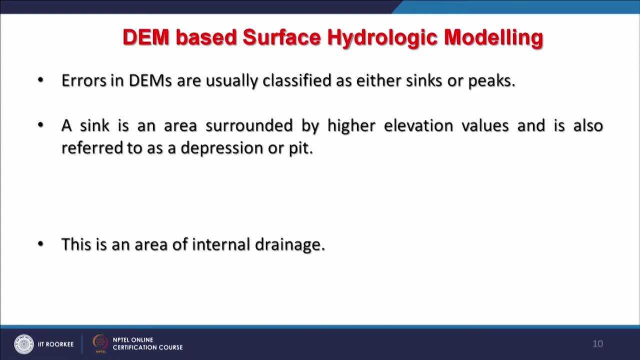 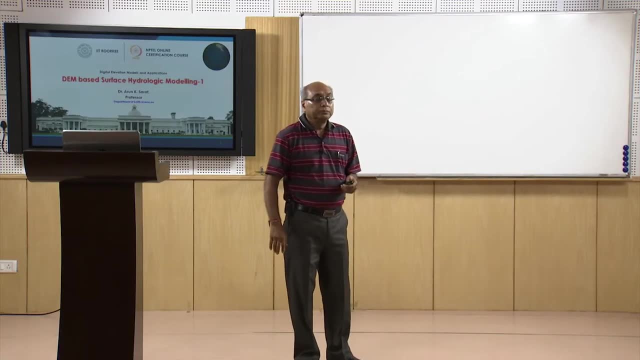 case of depression or in a peak it may be a lower elevation values. and this is the area of internal drainage, because here the surface runoff has to be there and therefore these have to be filled. And when the we are having a, When the we are having a. 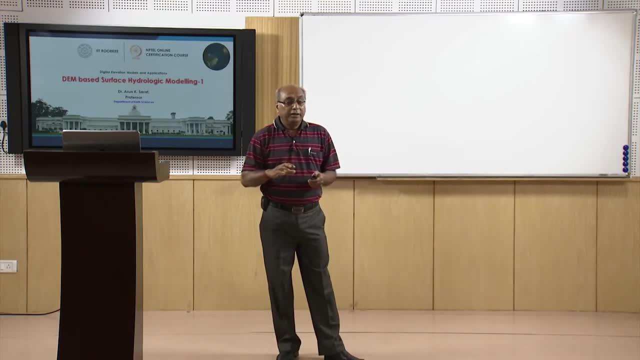 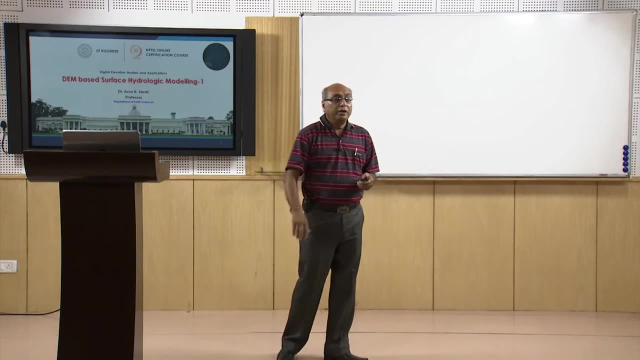 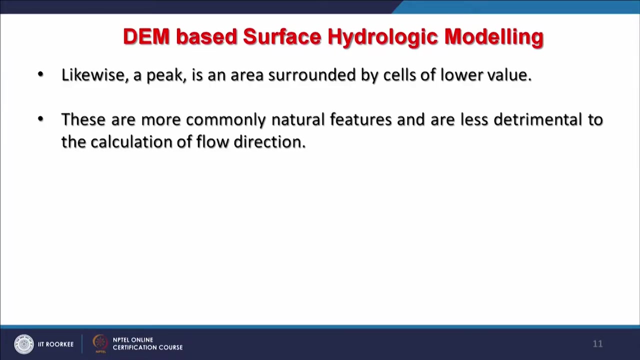 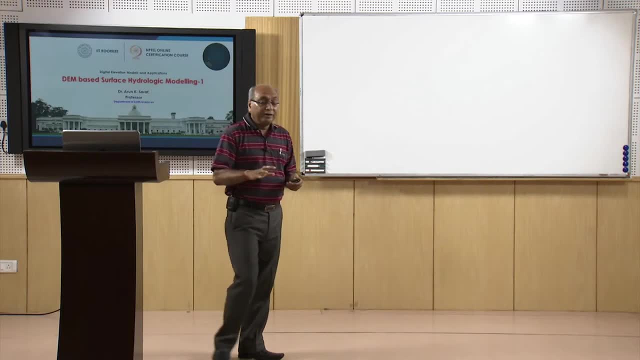 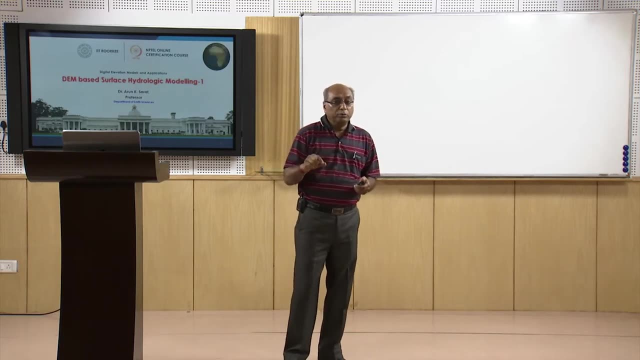 depending on the terrain and of course terrain ruggedness plays very important role, but the nonetheless these will be used while calculating the flow direction. So that is why in the flow chart, flow direction has been calculated first, but sometimes people first go for depression less. 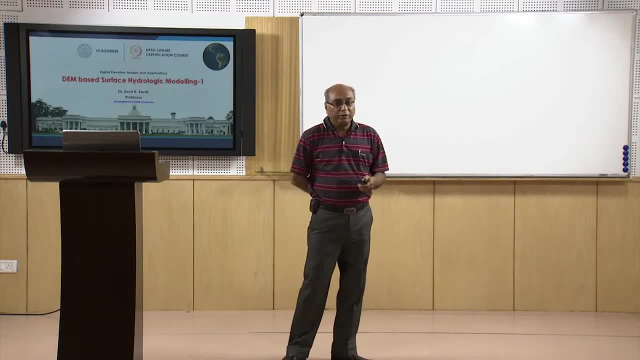 creating a depression, less TM, and then drive the other parameters. that is also possible. So these have to be removed or these have to be filled with surrounding values, and once it is done, then we assume that now water will flow over land or as a surface runoff And 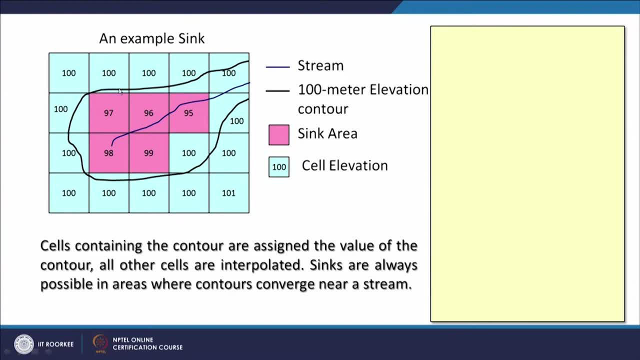 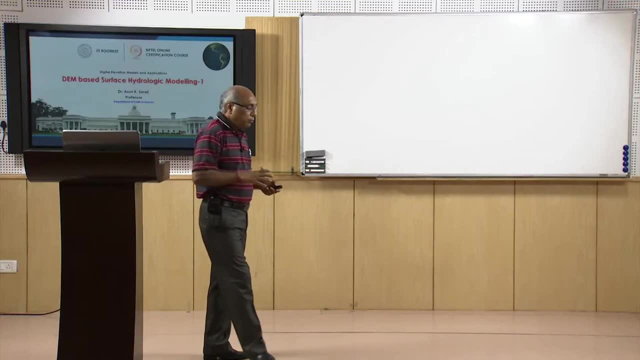 this is one example of sinks: here that there are 5 cells which are having values lower than the surrounding. So we can fill so that this depression is removed. But generally through my own experience I have seen the sinks are of. not that is my, 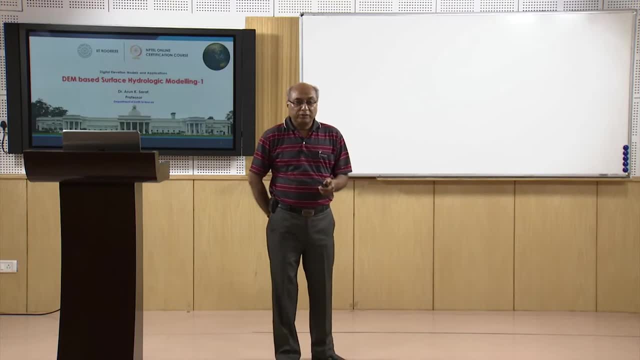 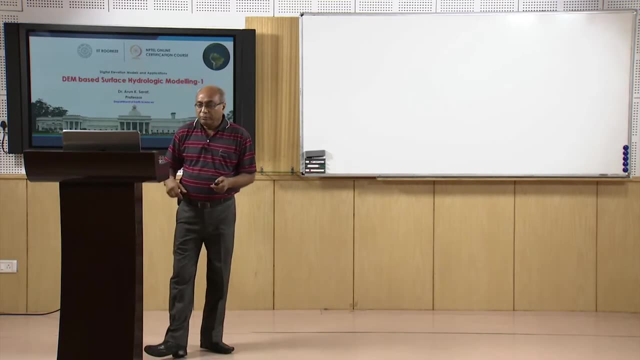 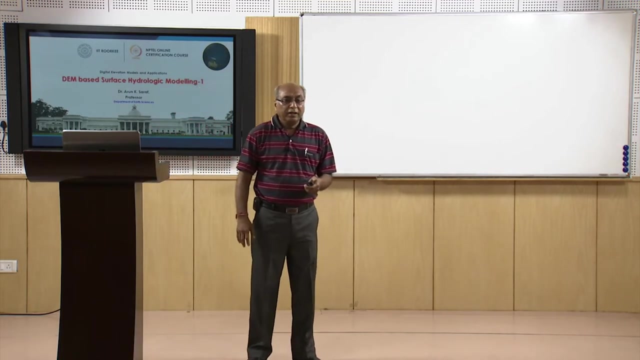 size. they are generally of just 1 or 2 pixels maximum and, as said that, the sink are the areas of internal drainage and we have to get rid of these internal drainage to allow water to flow over the surface. and these sinks can occur when all neighbouring cells are. 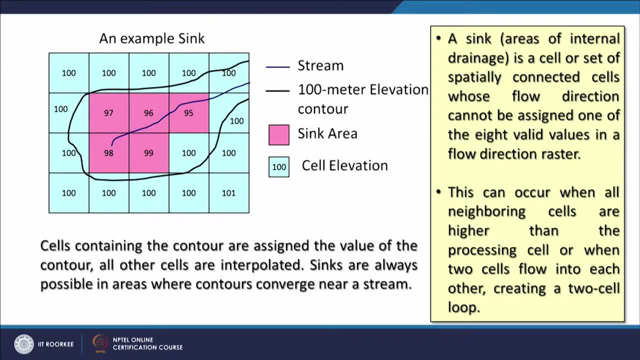 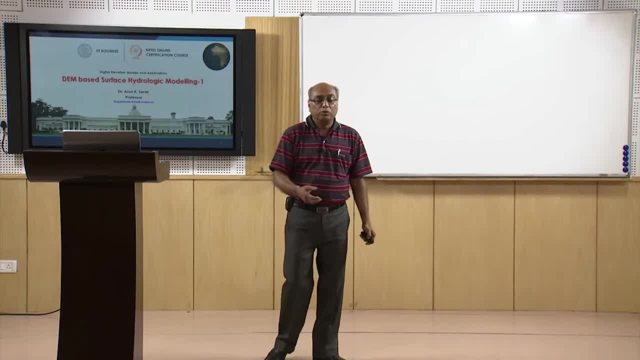 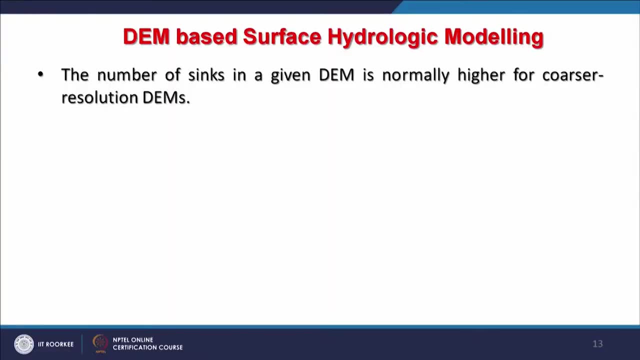 higher than processing cell or maybe lower in case of a peak in a sink. So this is a digital elevation model, but this peak is just 1 or 2 cell size, So number of sinks in a DM is normally higher. for coarser resolution: DMs because coarser resolution. 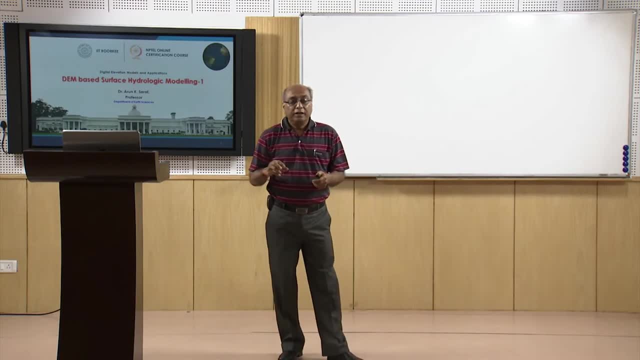 DMs may have more errors in form of sinks as compared to relatively higher spatial resolution. And now, instead of 90 meter spatial resolution, which we used to call as a coarser resolution, most of us have started using 30 meter or higher spatial resolution. So this issue of sinks have become little less or less problematic in our surface hydrology modelling. Another cause of this sinks results from storing the elevation data as an integer number. So by mistake, if data has been stored, then the because integer numbers will not allow the values. at least one least count will be there, and that is why it may create some sinks. So generally, as I have mentioned already that digital elevation cell values are generally stored as a real values rather than integer values, So this care has to be taken before. 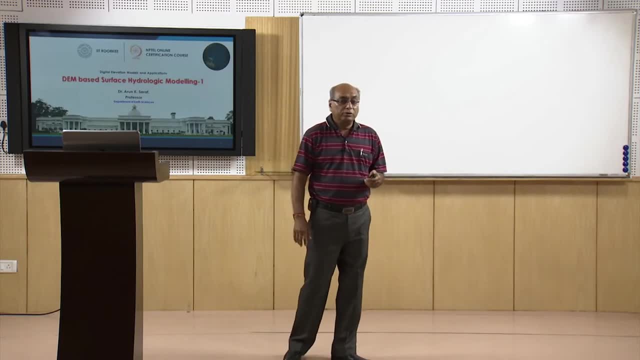 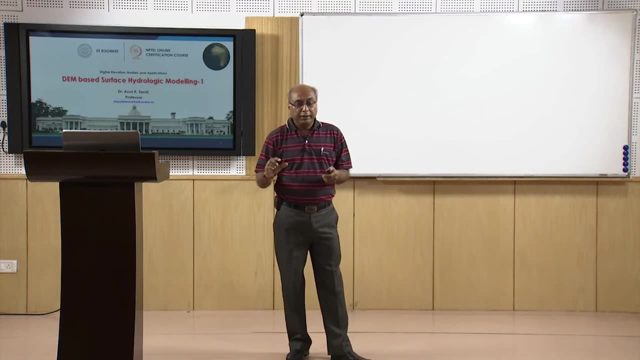 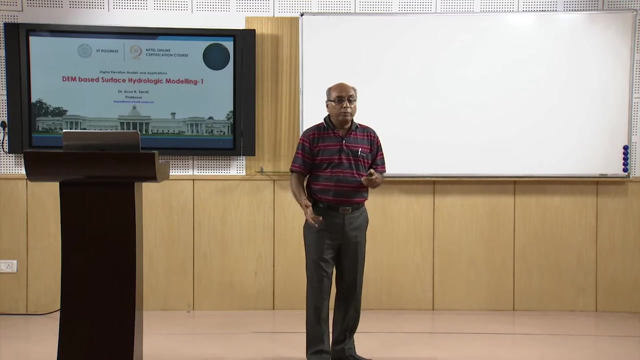 we put a DM through the surface hydrology modelling And as we know that these things can be avoided Once we get a digital elevation model of our area of interest, First we should study visually- otherwise look- the minimum values, maximum values and the cell values- whether 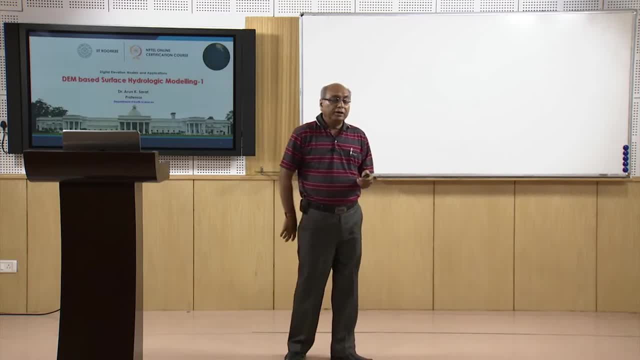 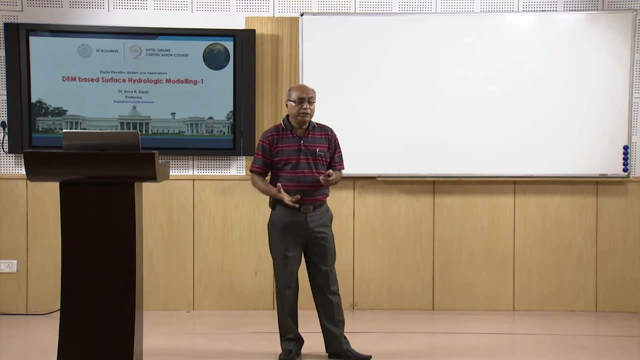 they are integer and real. once that is done, then we can proceed for surface hydrologic modelling. So depending on the spatial resolution, as in this example, as that in kbb is as much as 5% for a three arc set There. another issue is there is no sort ofке as we have. 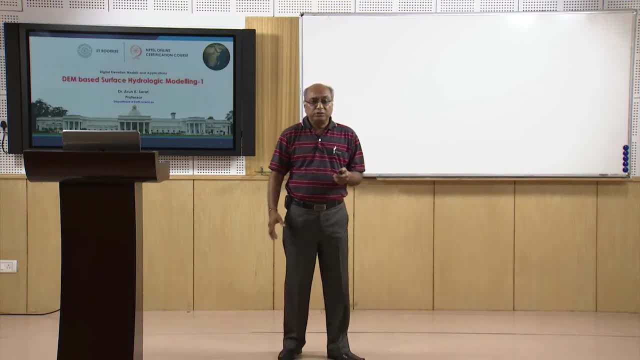 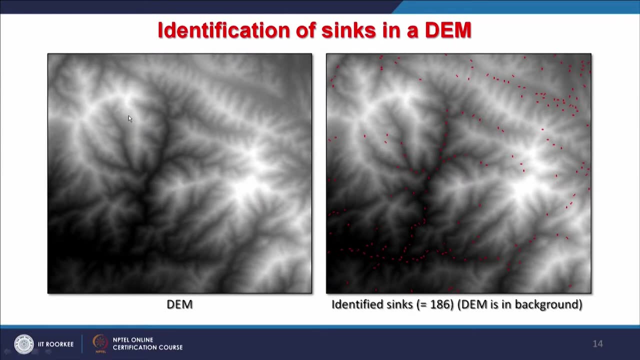 already? uh, within Kepler scale. basically, the verg is just a fixed set of values and deeper enemy values added to it. as another example, Have you considered these values for second DEM? that means 90 meter resolution DEM. The example is here that the same digital elevation model which we have been using throughout. 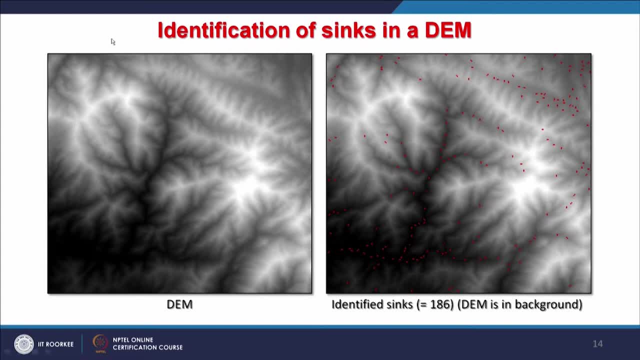 this course. the subset of that DEM is shown on the left side, and when this DEM was subjected to sinks or sinks identification, this is how these number of sinks have been identified, So the 186 cells which have been found having values lower than the surrounding values or 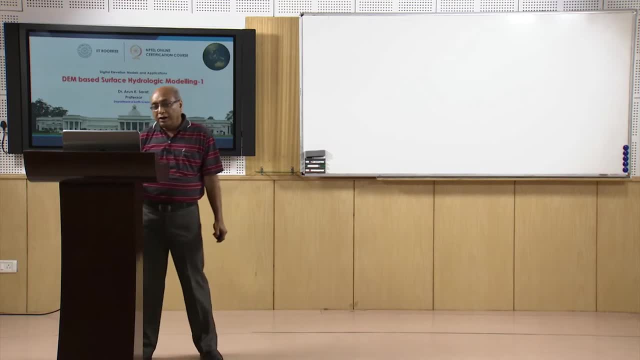 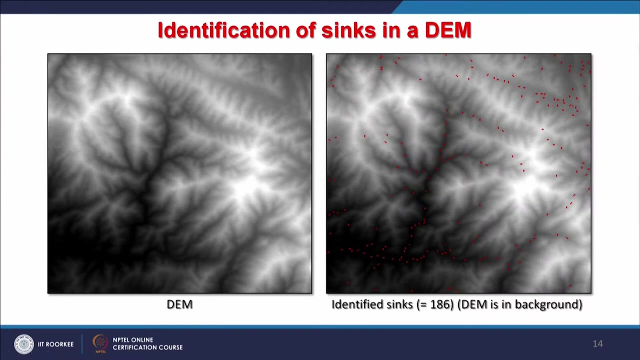 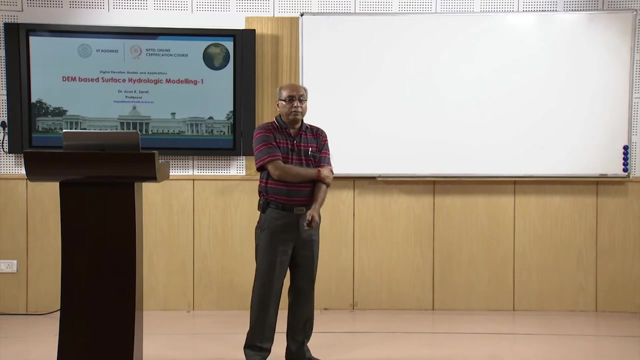 values having very significant higher values. So generally these are the depression, local depressions, which we need to remove or filled, and once that is done, then we can proceed for next step of surface hydrologic modeling. Now, so this analysis, or surface hydrologic modeling basically, is designed, the concept is based. 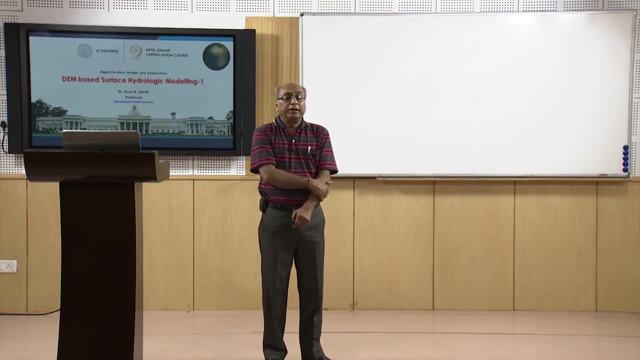 on this: the convergence of flow across a natural terrain surface. This has to remember that the water has to flow over the surface and this assumption, as I have been mentioning that this assumption basically, is that the surface contains sufficient vertical relief And that a flow path can be determined. 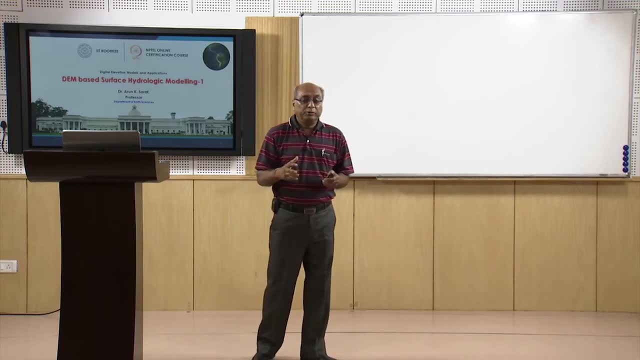 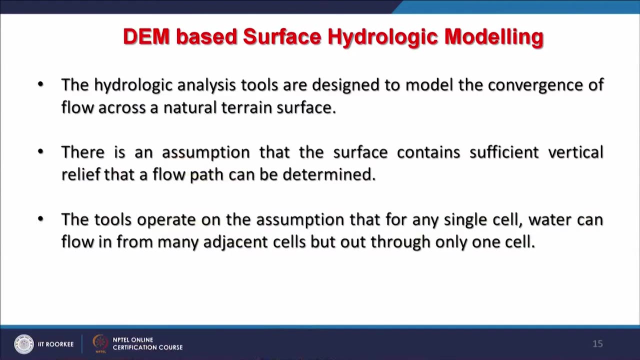 So you have to have a sufficient change in elevation and therefore, and the water can flow, and the tools which we use in different GIS platforms and they operate on this assumption that any single cell, the water can flow in from many adjacent cells, but through only. 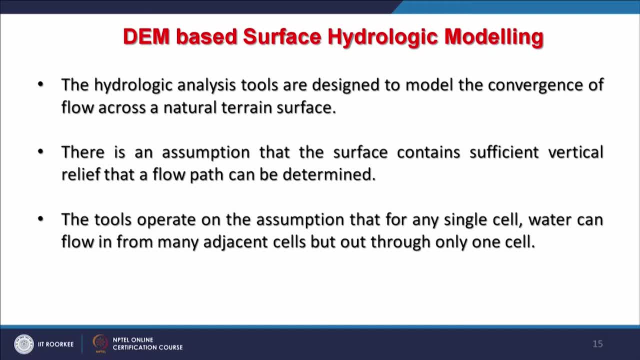 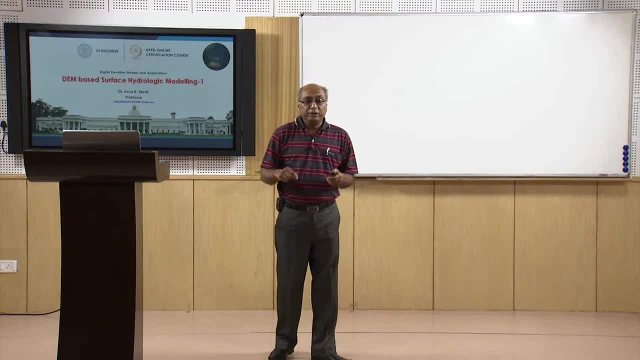 one cell. So there may be various cells, May be having lower value elevation values, but it will flow through only that cell, a single cell, which is having, among the surrounding cells, the minimum elevation values. And when we delineate these water sets or defining a stream network, we proceed through. 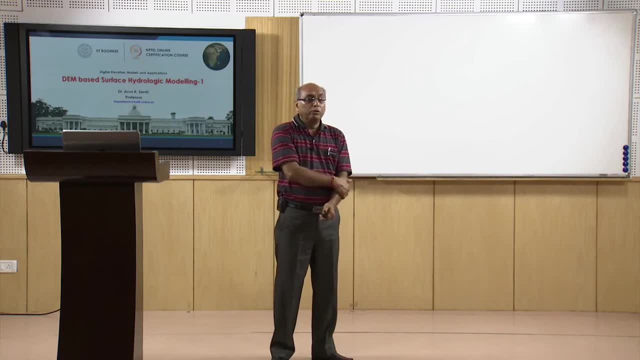 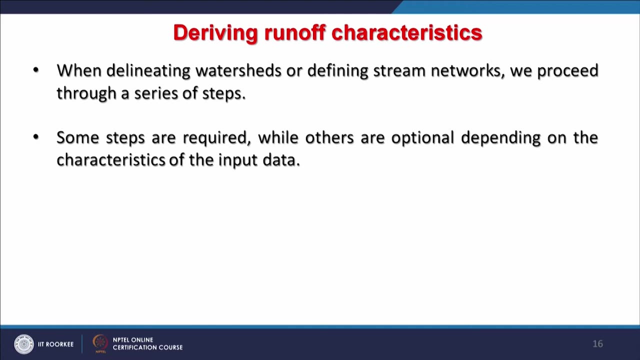 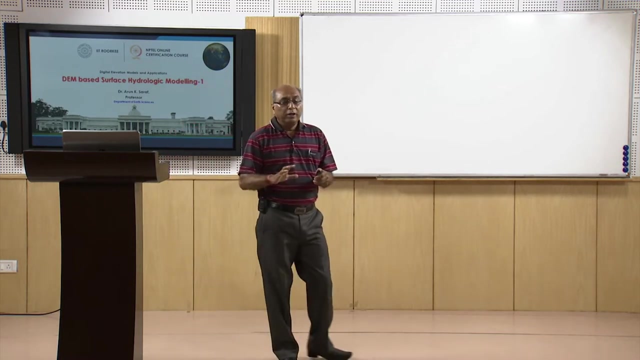 a series of steps as shown through the flow chart. Some steps are required, some other are optional, depending on the characteristics of internal input data and also depending on what we are going to achieve through this surface hydrologic modeling, because somebody may be looking only up to drainage network and not looking for 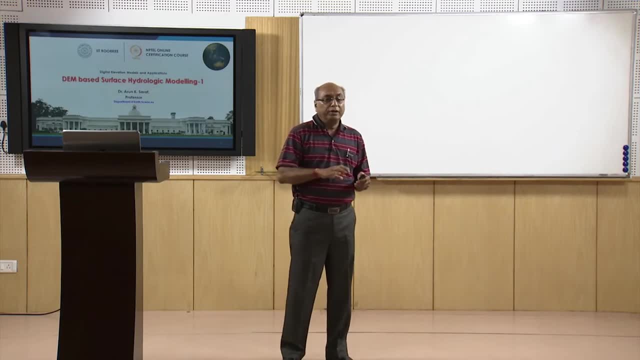 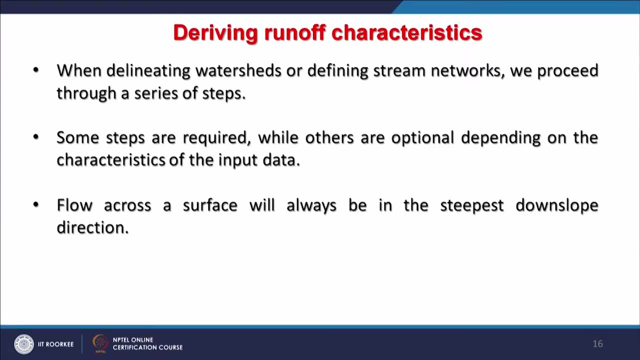 stream ordering or may not, be looking for water set boundary, So, depending on that, we go for steps, Flow across a surface will always be in the steepest downslope direction. This, we know, is a very simple, fundamental thing. So this is what we are going to achieve through this surface hydrologic modeling, because somebody 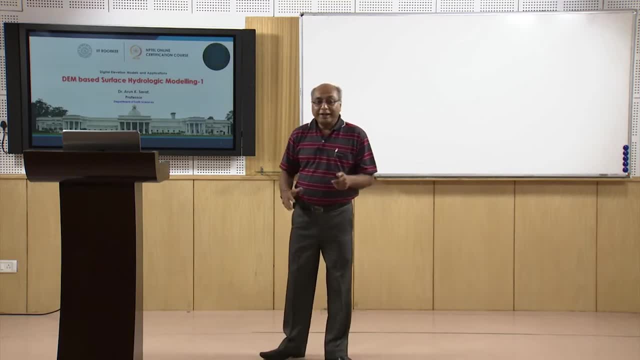 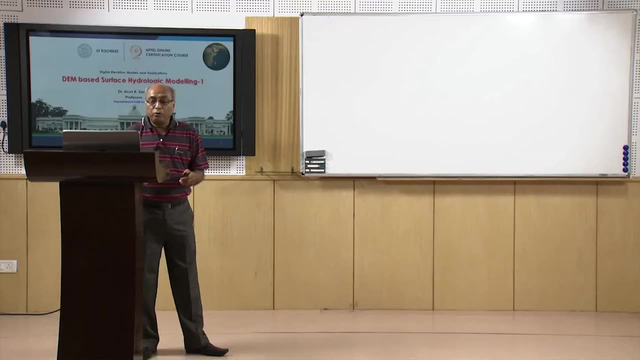 may be looking up to drainage network and not looking for water. set boundary, The basic thing once the direction of flow. that is why the first step here is to calculate the flow direction. So once the direction of flow out of each cell is known, it is now possible to determine. 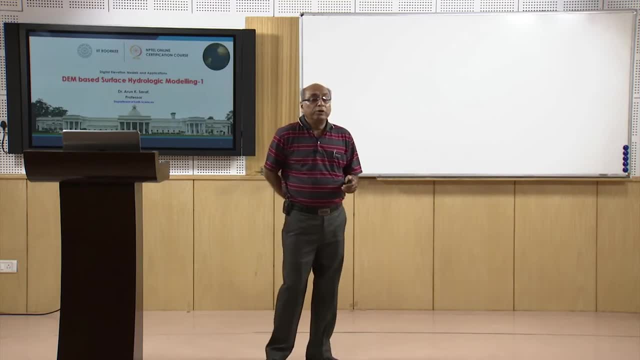 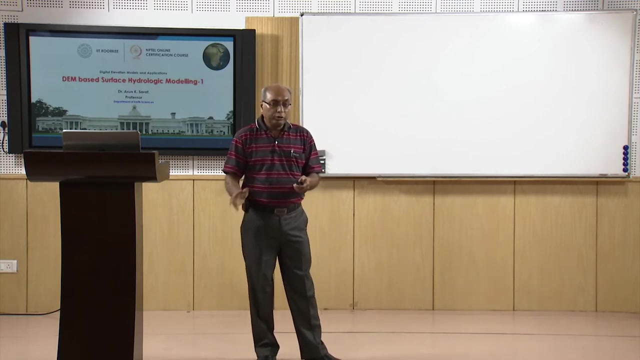 which and how many cells flow into that given cell, and that will decide the flow accommodation. So the first, after depression, that the Or even before that, the flow direction has to be calculated. So both approaches are available. based on the depression less or on the original DEM, the flow direction can be calculated. 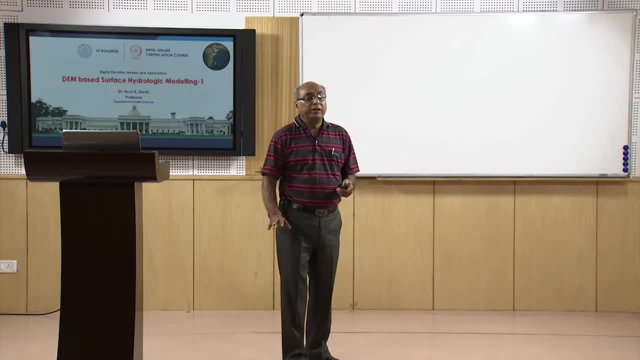 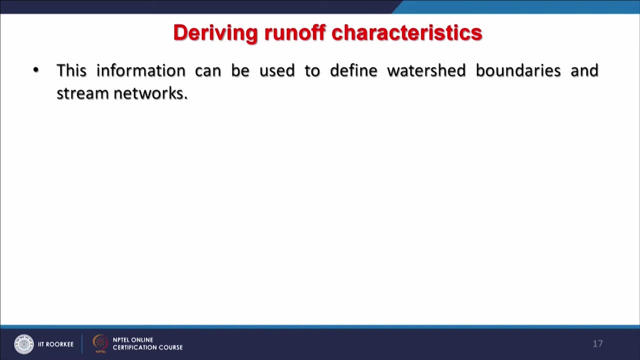 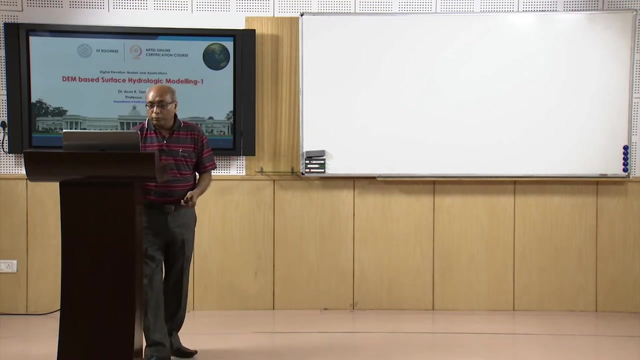 But for flow accumulation, a depression, less DEM has to be there And the information can be used to define water set boundaries and stream networks. that is the flow accumulation information And these, the chart which I am going to show, are having this information: water set, boundary, stream networks from a digital elevation models. And we start with. 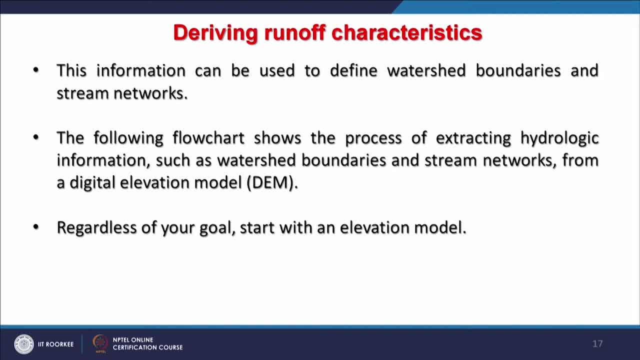 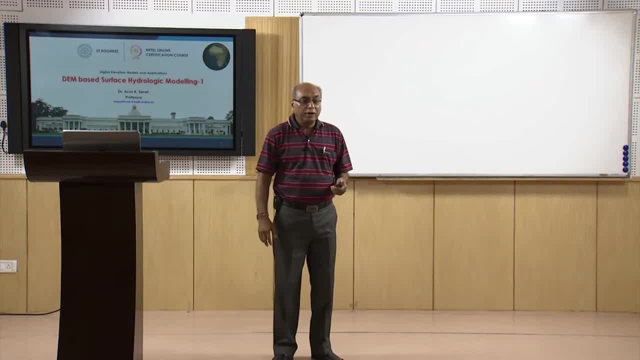 always, whatever is the ultimate aim or ultimate derivative which we are targeting, we have to start always with the digital elevation model And this is based on in which cell The water will flow, from which cell and this will decide basically the direction. So this: 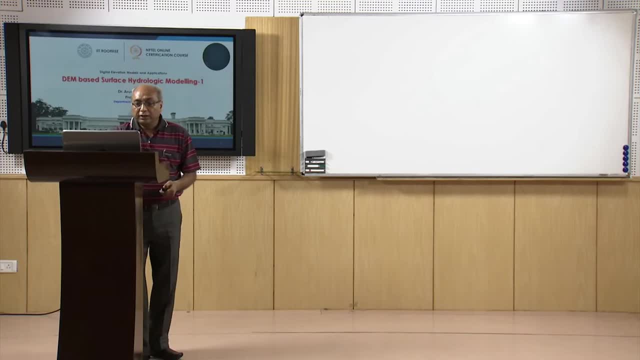 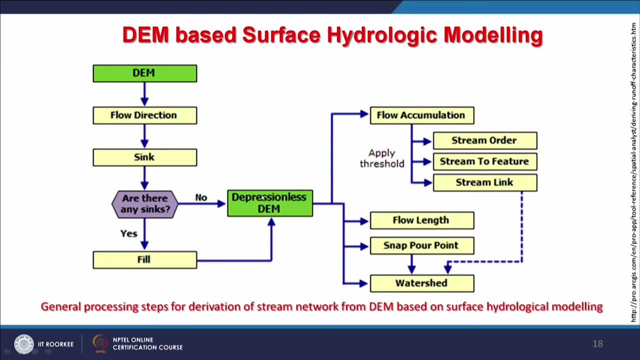 is a repeat flow direction, that flow chart which is here that we will, after having a depression, less DEM, then a flow accumulation theme is calculated. This theme, as mentioned, can be used to drive a stream network, stream order or stream to features means from raster to vector. 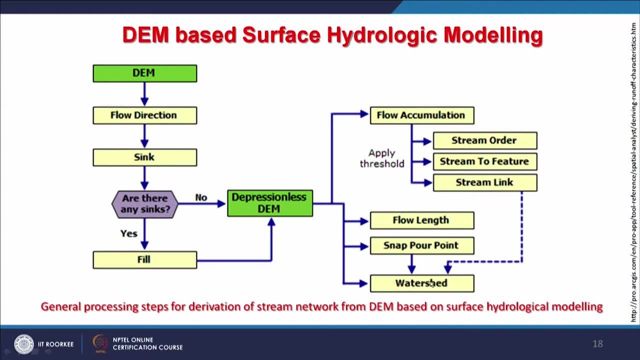 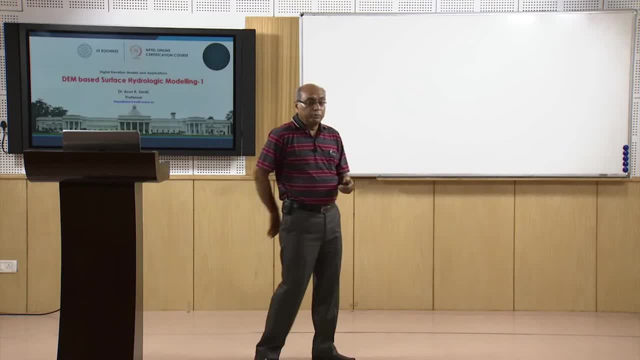 Here or a stream link files which can be used later on in case of water, set boundary delineation and other in between parameters can also be drive, So like driving runoff characteristics of from of a DEM, of a terrain through a surface, ordinary modelling. So the error part we 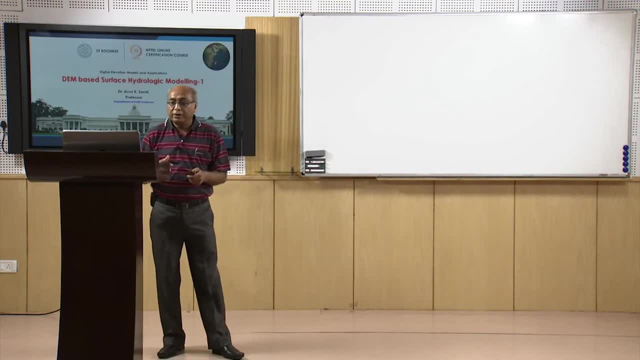 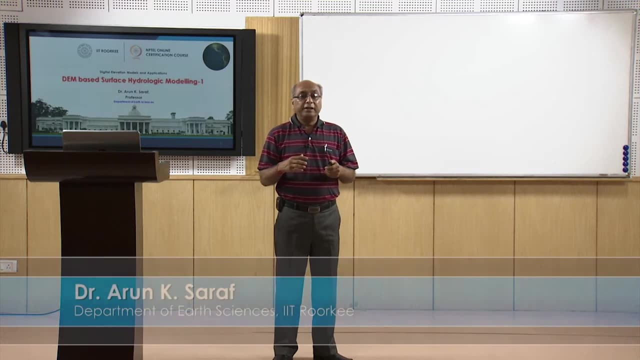 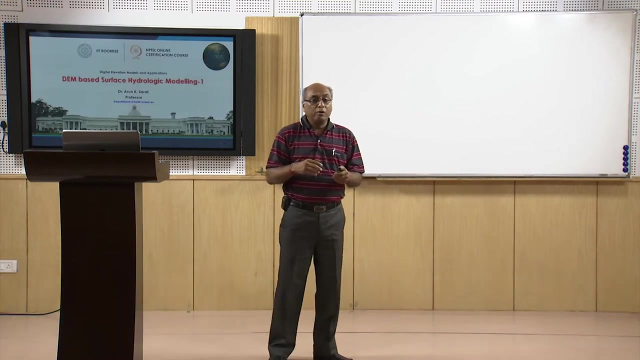 have already discussed that if there are errors in digital elevation model, Or if you are modelling a cost geology, that means the and the terrain which is representing a limestone terrain. and you know, there we are having these limestone related lock rocks and then one has to take care because we may have a large sinks there. 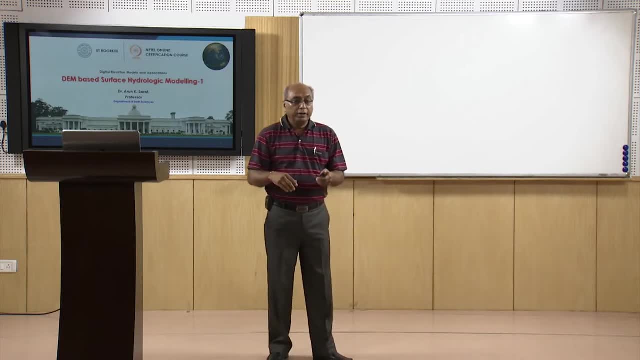 Otherwise, generally we do not have this problem And so they, because you may have these lower areas. Okay, And generally in this cost topography or cost geology, we do not have this. in calcareous terrain we do not have surface drainage, So only subsurface drainage network is there. 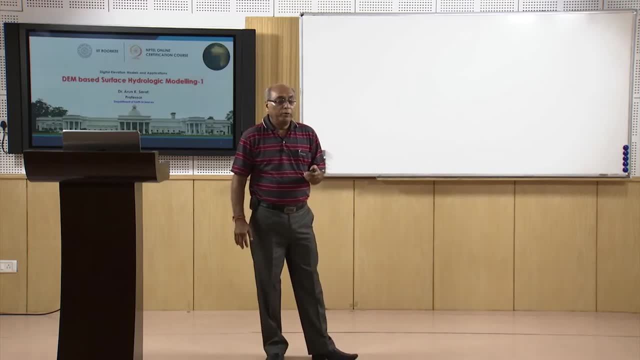 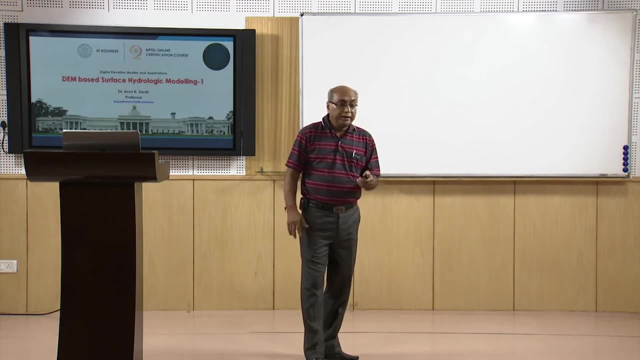 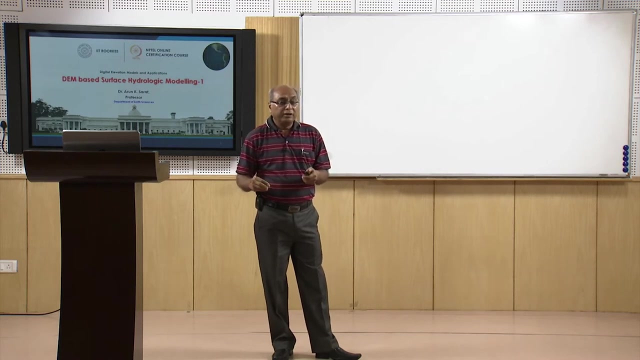 but it is a very, not a common phenomena. And if this is the situation, then then probably the surface hydrologic modelling will not work. But otherwise, in most of the cases there is, should not be, any problem about this. So when we go for depression and remove the depressions, or depression less elevation model, then we 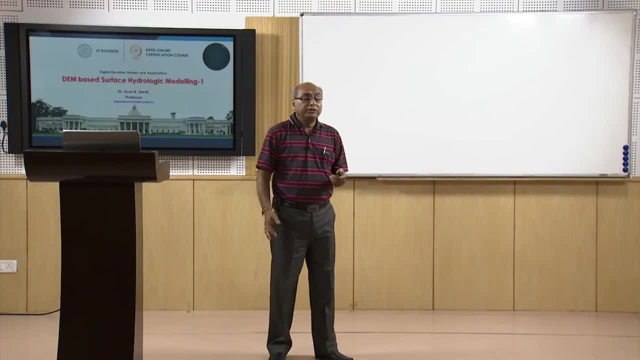 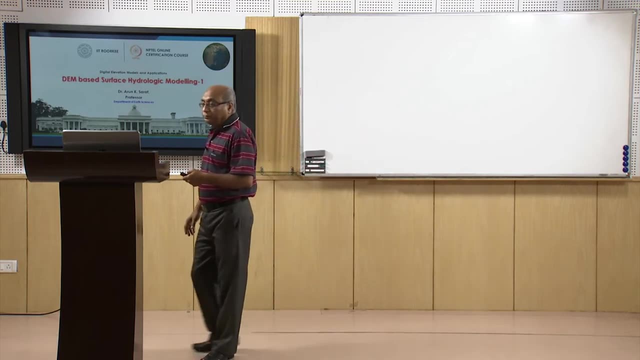 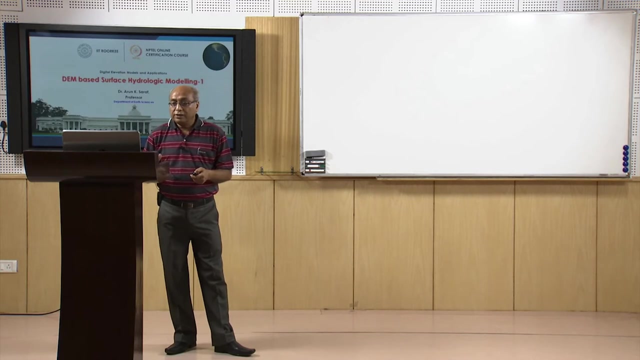 can also later on drive the flow direction, flow flow accumulation and so on, so forth. While delineating watershed boundaries, first 4 points need to be identified. First 4 points need to be identified that we have already discussed. Then these locations are mouse: 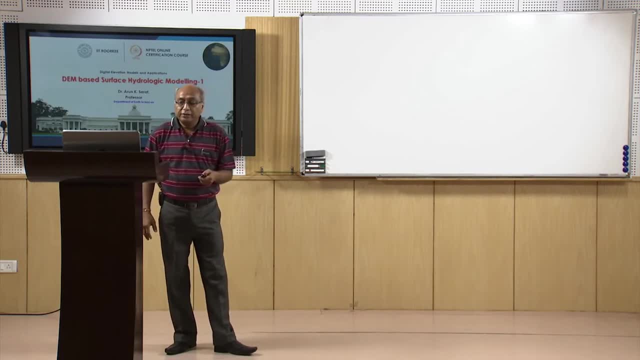 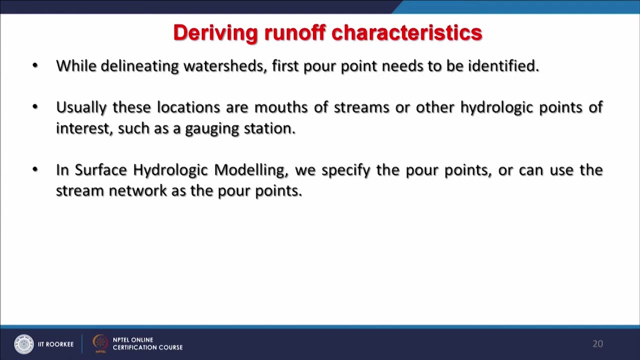 of streams or other hydrologic points of interest, such as gauging stations, And in surface hydrologic modelling we specify pore points while delineating a watershed boundary, And one can use the size of, give a threshold, that if 500 cells or 5000 cells or a square 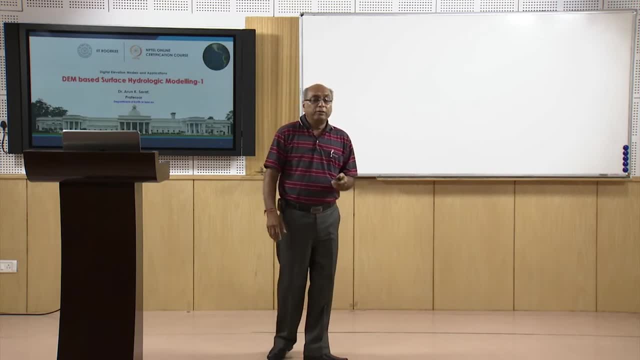 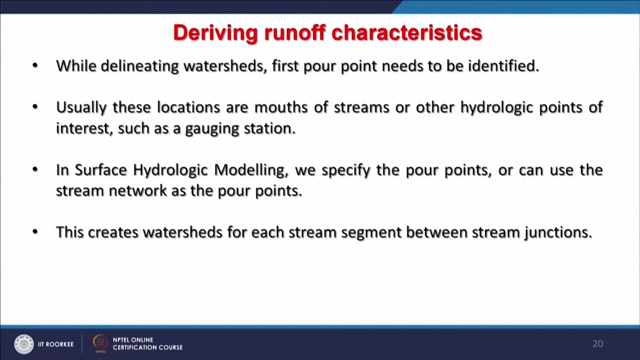 meter area is contributing, then I want to delineate So likewise the drainage network and everything can be determined, And this to create the watershed for each stream segment between stream junction. So stream link information is also becomes very important. Once the drainage network has been derived, then we can use. 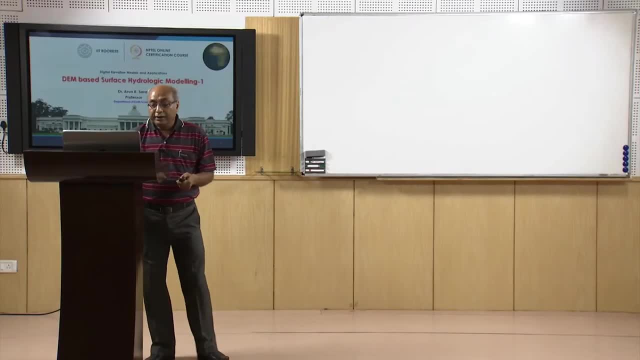 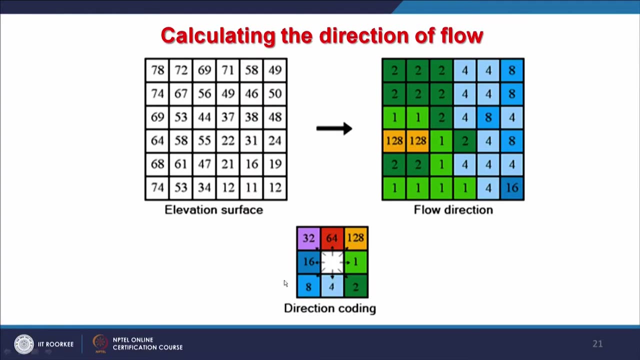 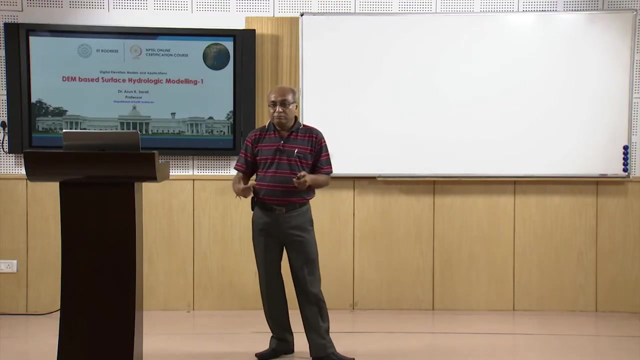 for other things. So, in order to create a drainage network, after the flow and direction, next thing is flow accumulation for each cell is calculated. If we look on the cell basis, how flow direction the one major theme which we drive is, so on. 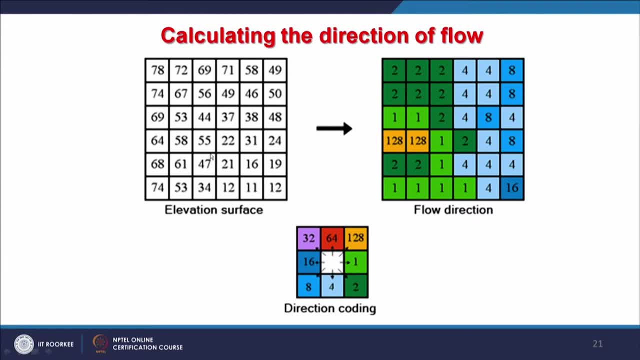 the left side, top left. basically, we are having a digital elevation model of a very small area is shown here, And when we create a flow direction, we follow a scheme. Generally, this is the scheme for coding, So these are not basically elevation values. these are: 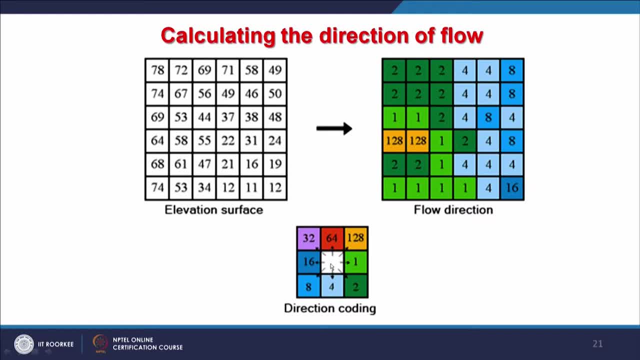 the codes of flow direction. So when a cell is allowing water to flow towards the east, then the code 1 is given. When it is going for southeast direction, then code 2.. Likewise, when it is going for north direction, then code 64 is assigned, and if it is going to 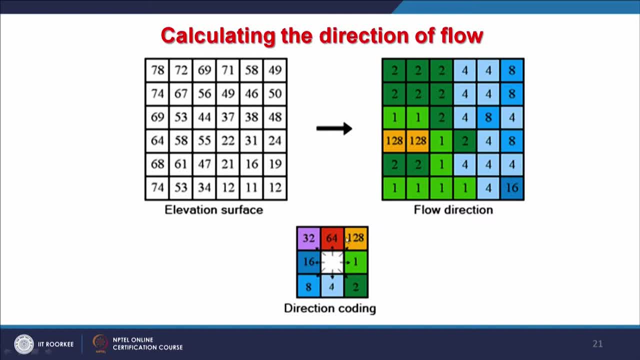 going for northeast direction, then 128. So it is in a particular digital elevation model. may not be necessary that all codes will be used Same thing here. in this example there are few codes, like in the 64 code, 32 code and. 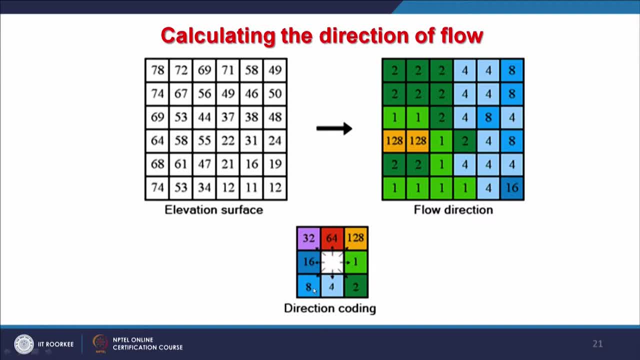 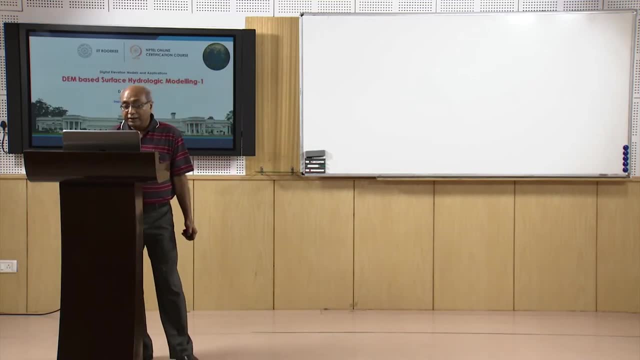 these codes have not been used, whereas code 1, 2, 4 and 128, 16 have been used. That means the flow in these directions. within this example, DEM are there, but in other directions, like in north direction, northwest direction, there is no flow is there? So it is not necessary. 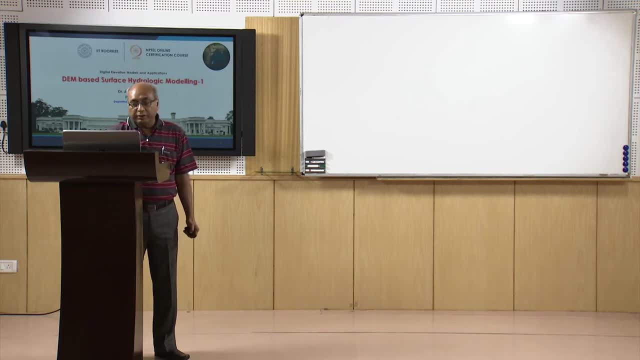 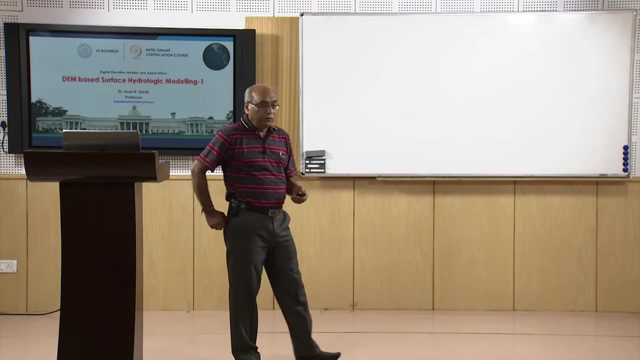 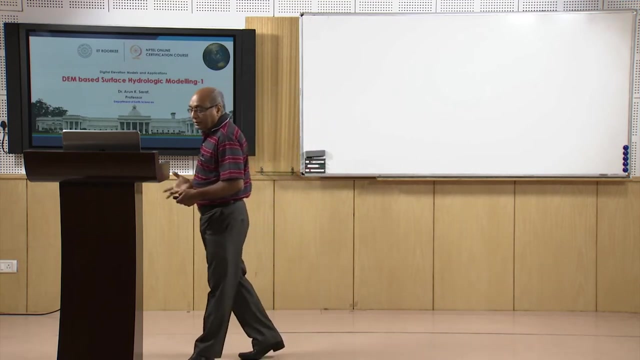 that all codes within a given or as a DEM will be given. these all codes there depends on in which direction the flow is going to flow from. water is going to flow from one cell to another cell, So flow direction. conclusively, a definite line or codes in which something is issuing. 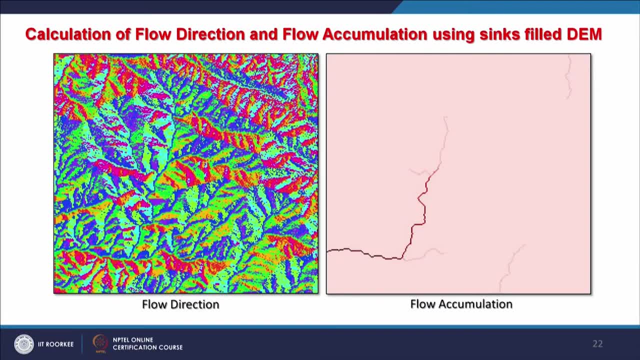 or moving in a stream And when we see in a form of the same digital elevation model and really large file instead of just on cell based, as we have been seeing in previous slide Here. this is the DEM. We have taken an example DEM throughout this course and the flow direction has been determined. 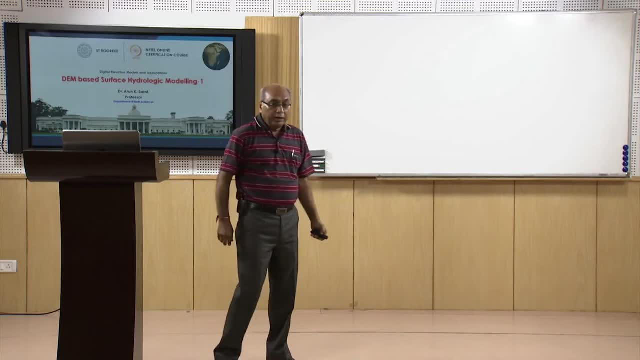 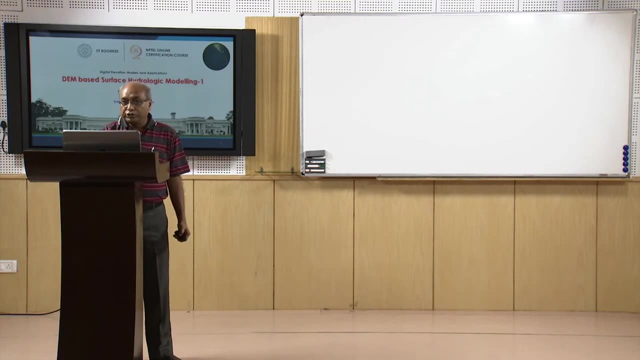 Sometimes one may feel the flow direction looks more close to slope map. In fact, yes, in some way. but basically the codes have to be taken care, because the codes there are different than here. otherwise the output may look similar in that sense. But we cannot equate. 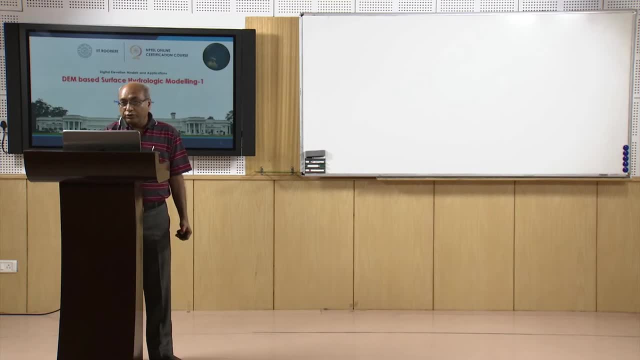 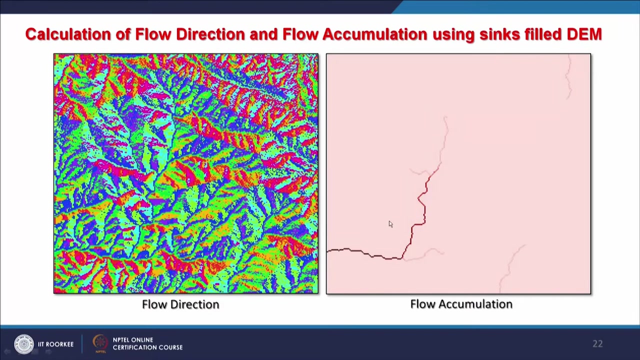 it directly, So codes have to be taken care, because these codes are later on used while calculating flow accumulation. So this flow accumulation map is here, So this is showing the major drainage and, of course, on a GIS platform, if I click directly, say here, then 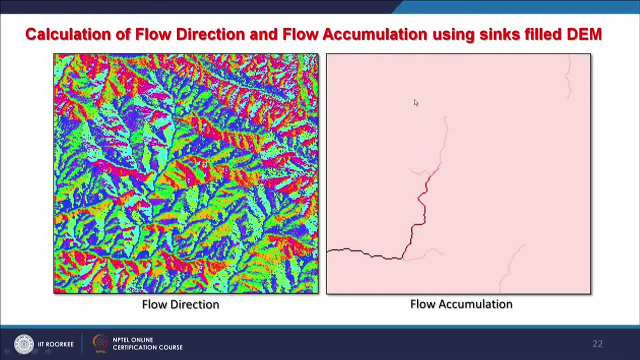 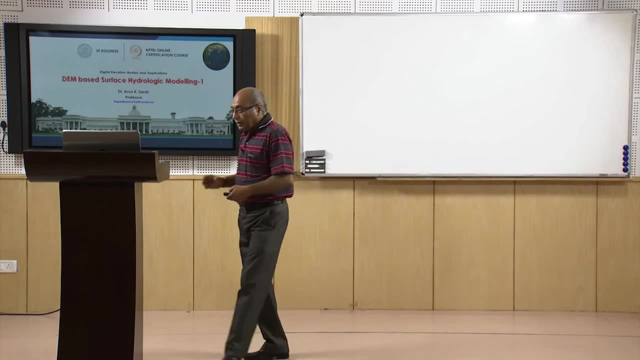 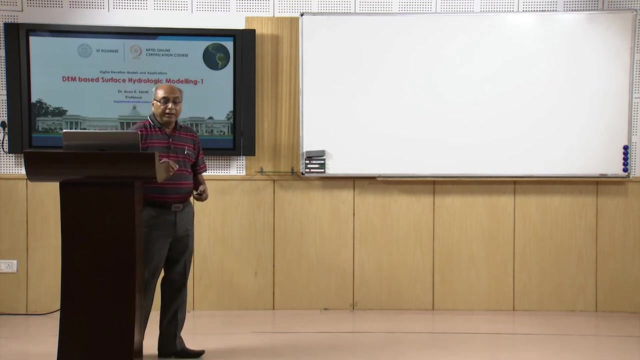 automatically a watershed boundary will be delineated. So they say this: flow accumulation, flow direction and flow accumulation generated using a field, DM. in this particular example Now, how to identify stream network? For a stream network, the theme which will go as a input is, of course, the flow accumulation theme, and here it is that we have to define. 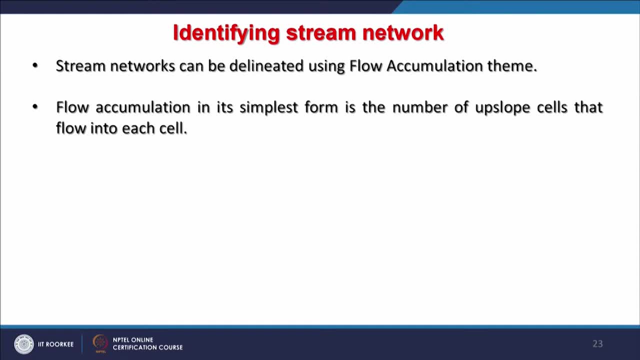 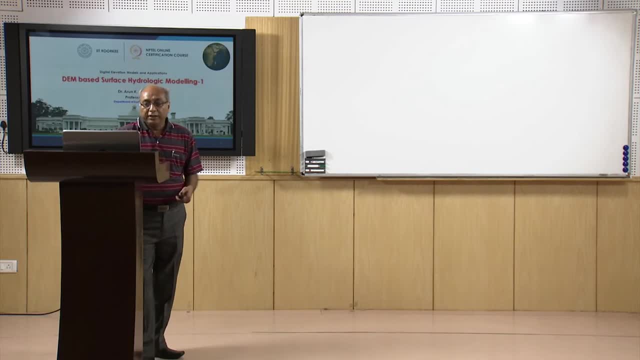 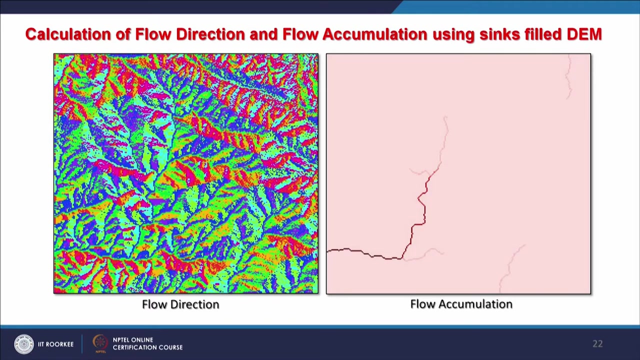 will be different. So flow accumulation in its simplest form is the number of up-slope cells that flow into each cell. So if I take an example here at this location, the maximum number of cells will contribute at this location. But if I go here then relatively over here. 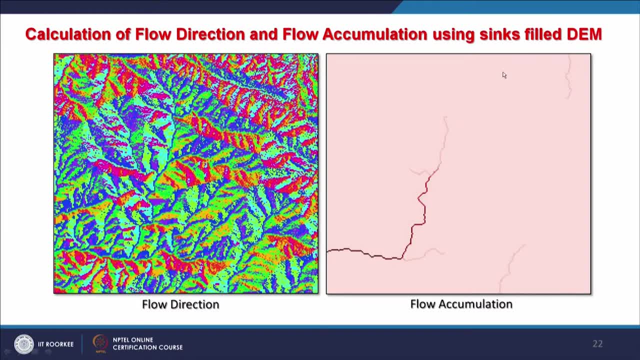 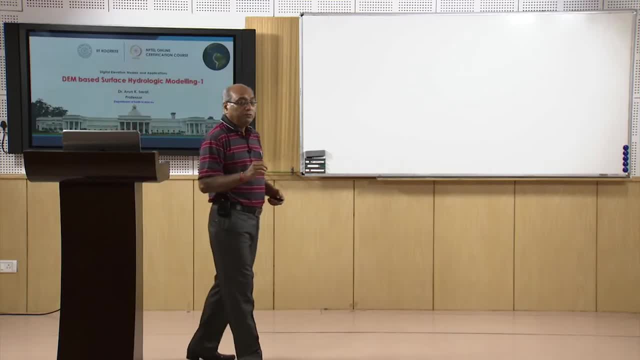 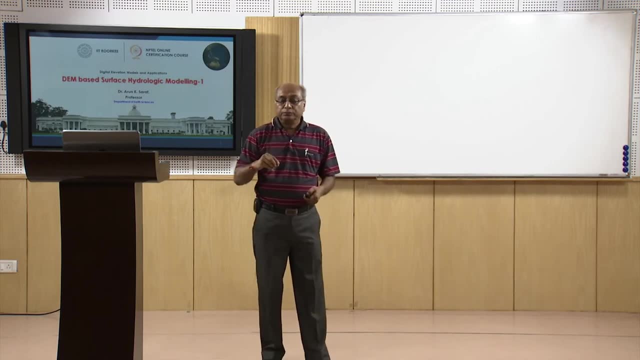 I will have less number of cells which will be contributing at this poor point. So this is what it is meaning is that the flow accumulation, in a simplest form, is the number of upslope cells that flow into each cell, and therefore the values will be also accordingly. 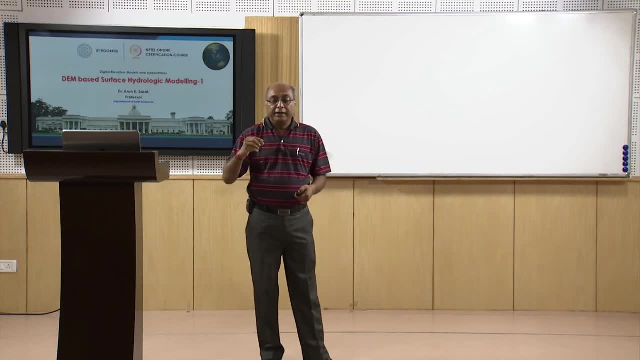 So at higher elevations, say near water set boundary, you will have a very small flow accumulation value, whereas at poor point or at the, in this particular example, at the edge of our water set, from where the water will go out of my study area, the flow accumulation 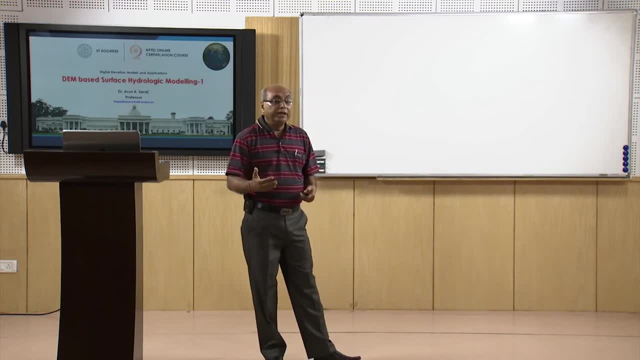 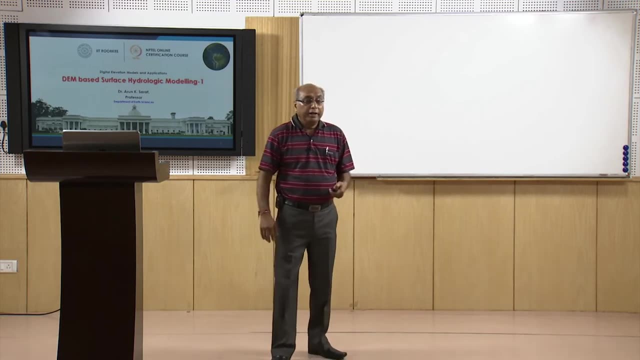 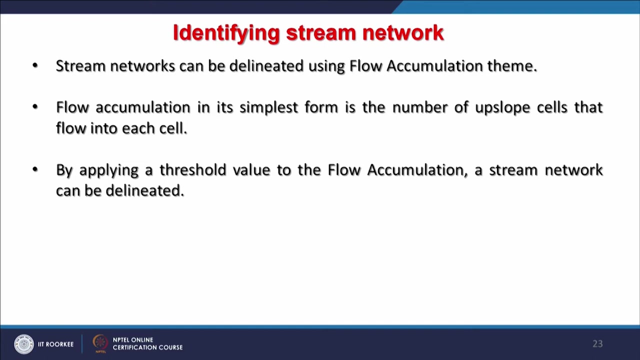 value is going to be very high because it is declaring the upslope cells which are which are going to flow into each cell. And by applying this, a threshold value, to a flow accumulation theme, a stream network can be derived. And likewise, I will just show you that, for example, if I to create a raster where value 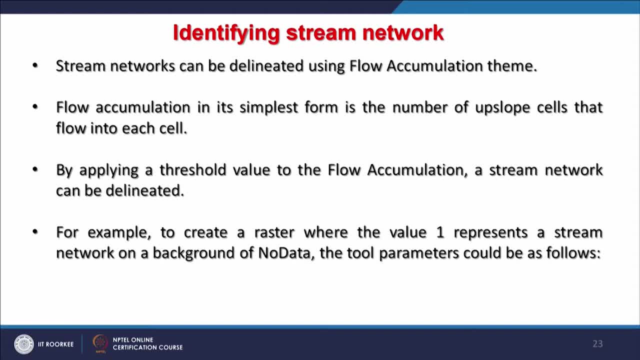 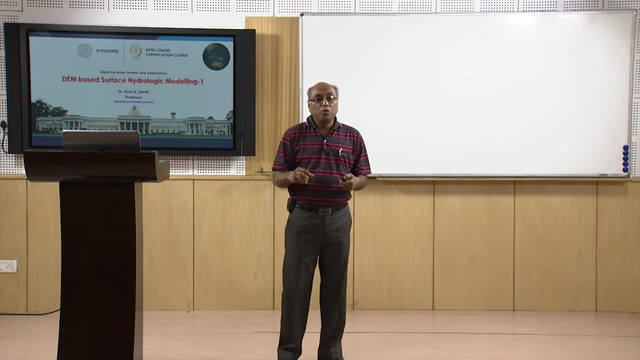 1 represents a stream network on a background of no data. the 2 s parameter could be as follows: that, for example, I can decide that the threshold value is more than equal to, say, 100 cells. that means that if 100 cells or more are contributing, then start delineating. 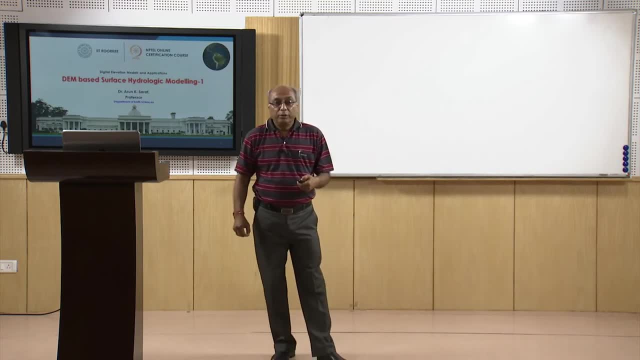 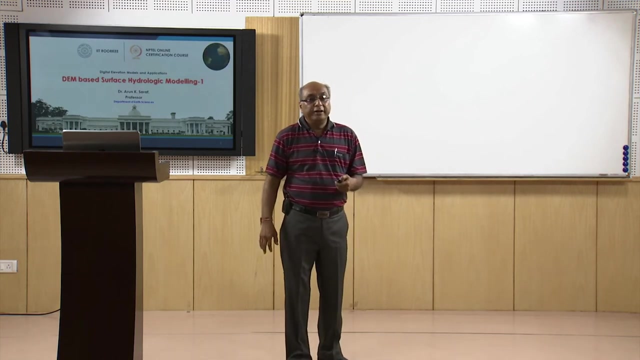 drainage network from there itself, because I cannot have one each cell. if I go and reduce this value, then 2 dense drainage network will be delineated which will not be close to natural drainage network which we see on the ground or through a topographic map. 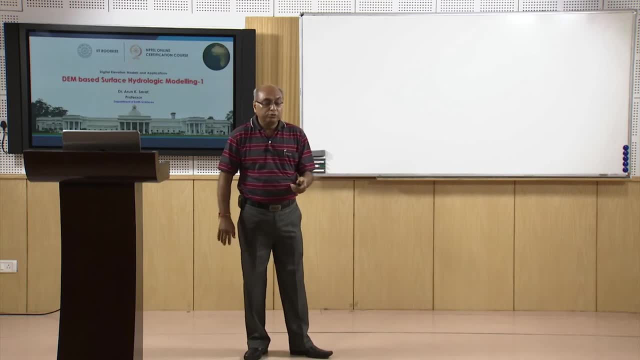 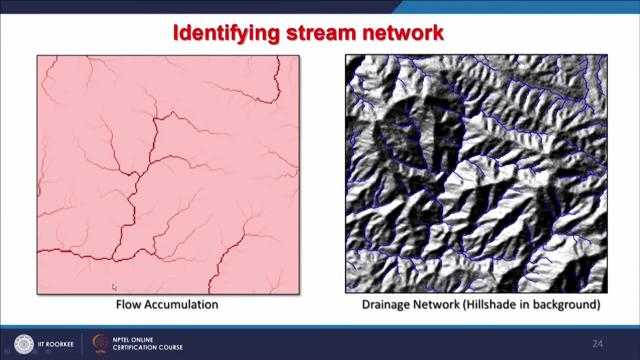 So this threshold value has to be judiciously chosen so that at least some comparison can be made. So here, flow accumulation is there and what we are seeing here: the drainage network in form of blue lines, and in the background, a hillside has been put here, just to show. 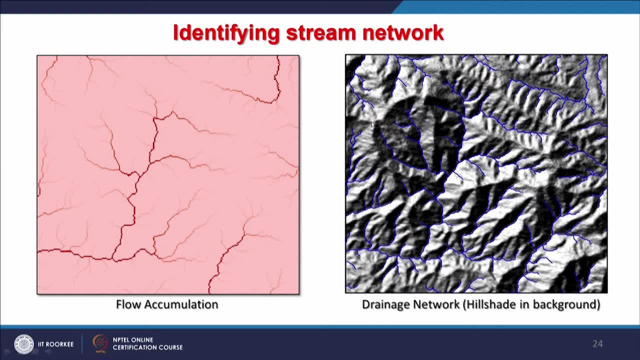 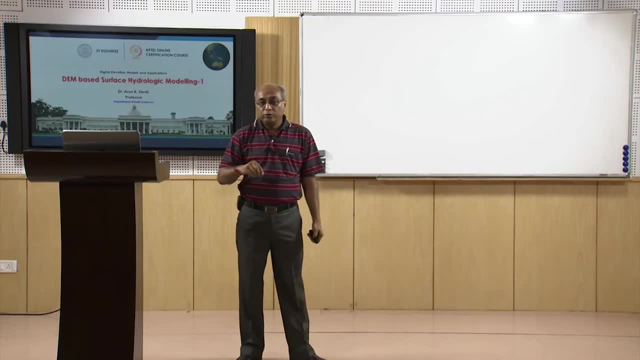 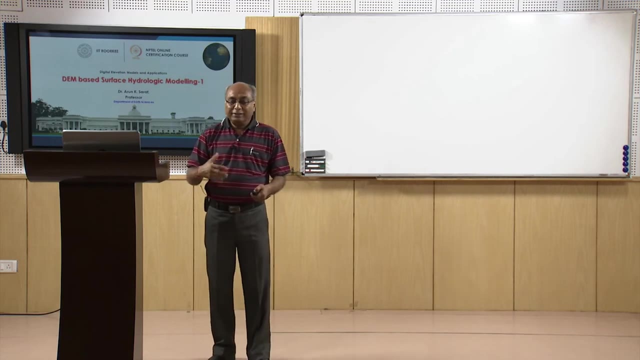 that how, if this becomes the watershed boundary and at this outlet, as you can see, and the drainage is just going through here. likewise, If I have chosen a very small value as threshold value, then too much drainage lines would have been delineated, and though the system will calculate, but they may not be close to. 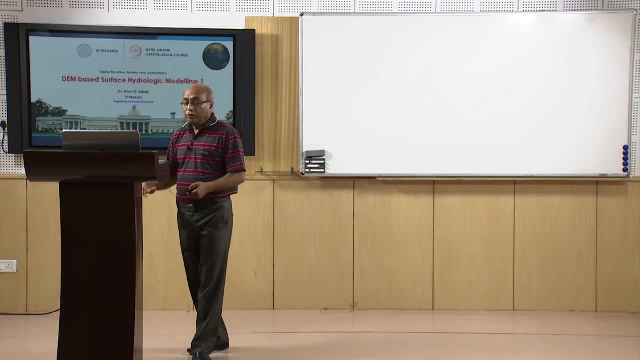 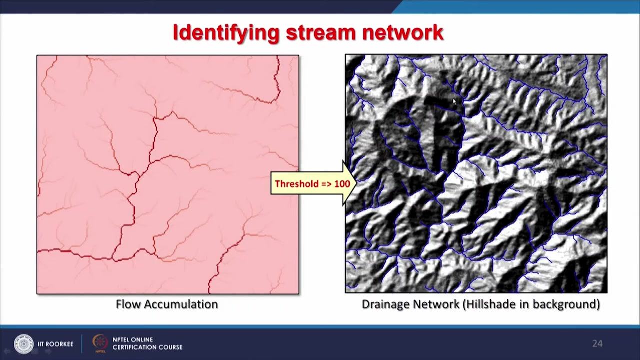 realistic means you will not see on the ground really, or even on a large scale topographic map. So it is always one has to be careful while choosing the threshold value. So here, In this particular example, the threshold value was equal to a greater than 100 cells. 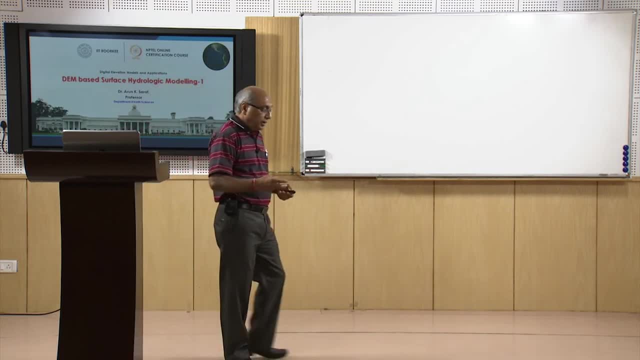 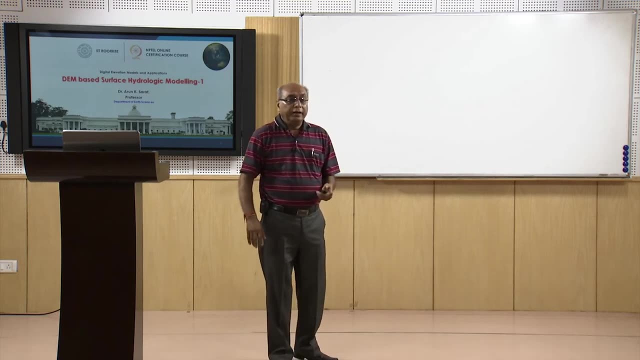 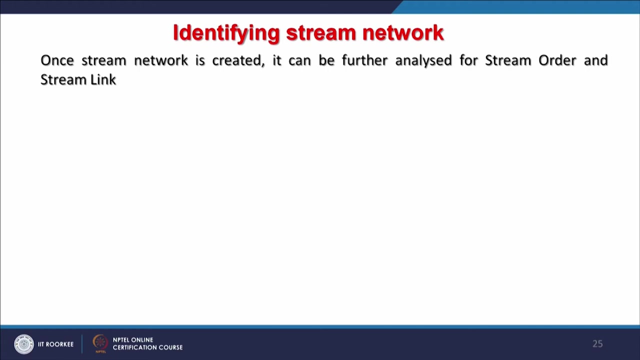 So once we choose the or one may go for, instead of number of cells, one may decide based on the area and accordingly it has to be given. Once the stream network is created, it is further analyzed for stream order or stream links. So, as I mentioned in the beginning, that is a you know. 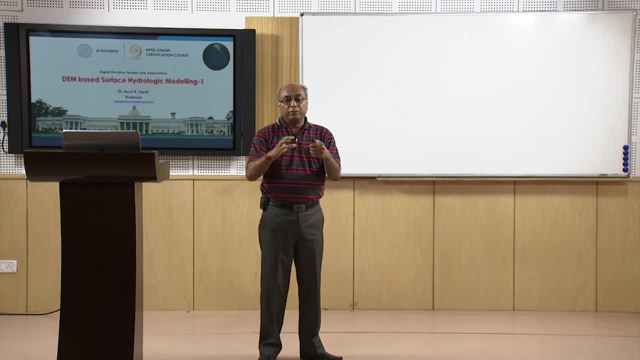 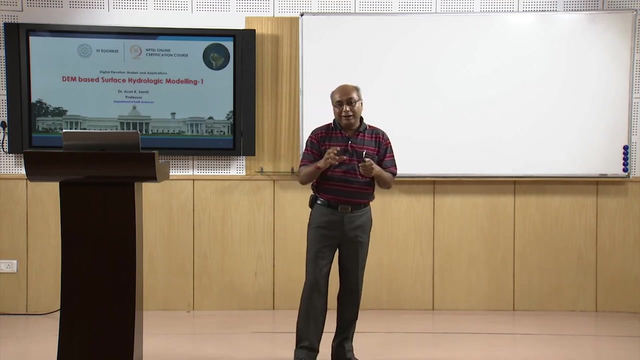 Sequential processing. we started with digital elevation model. we filled the depressions, we calculated the flow direction, we calculated then using the flow direction, we calculated the flow accumulation. Once the flow accumulation is there, we apply a threshold value and calculate it and determine. 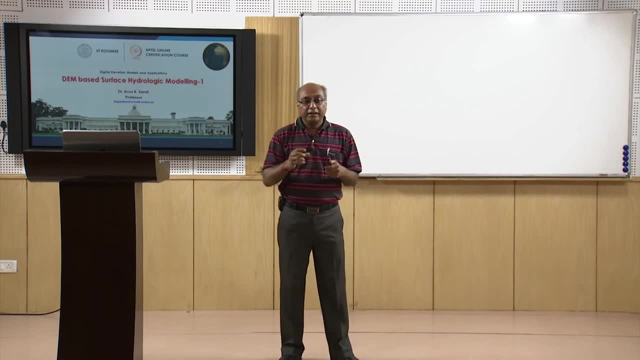 the drainage network. Now, once drainage network is there, then this we can use to drive two products. One is stream order and stream links. Stream links is used, Stream links is used later on, but stream order- there are different stream schemes which exist. 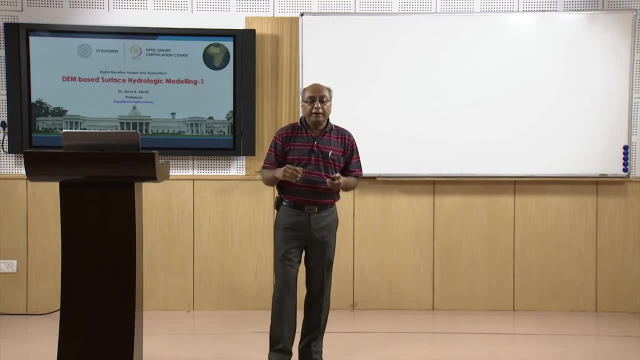 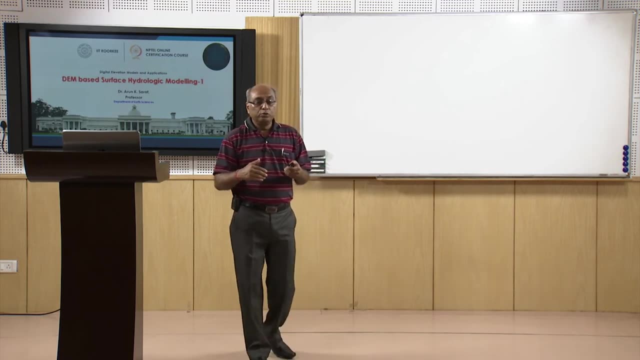 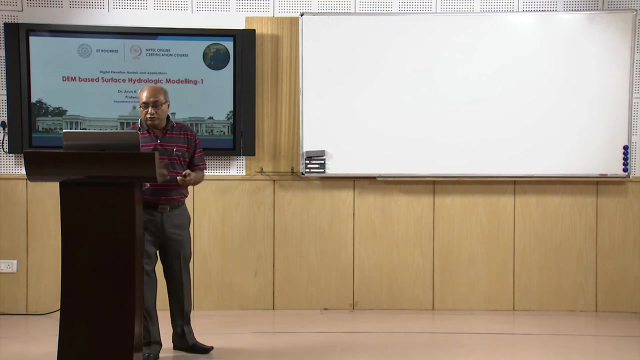 The most popular one are the SHRIB- given by a scientist or geomorphologist- SHRIB and STELR. So these two stream ordering schemes have been implemented into GIS softwares and, within this surface hydrologic modeling, And there are slight changes in this. we will see the differences in this. 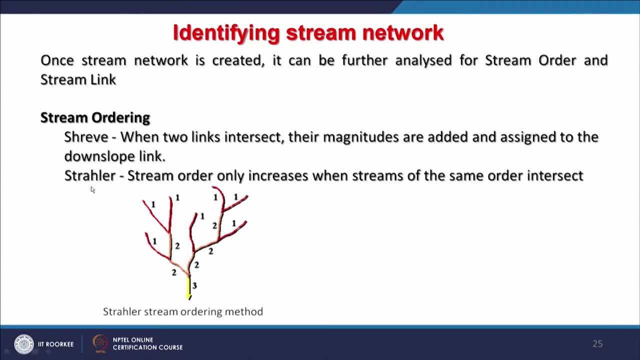 That in this STELR. let us take the later one first. So STELR stream order only increases when streams of the same order intersect. What does it mean That when I am having order 1,, first order stream, first order stream, when these two 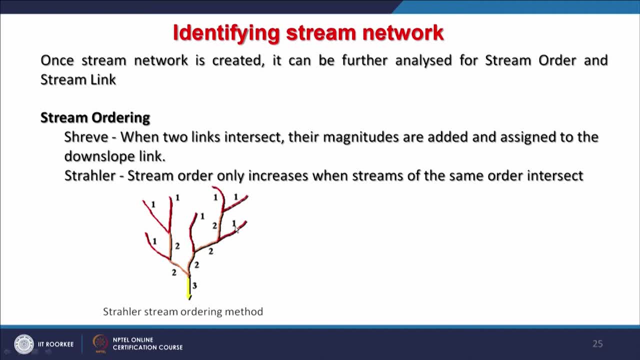 meets, then it becomes second order. When second order and first order meets, then still it remains second order. So this is the first order, The second order and first order. So this is the first order. So once we are having two second order streams, then only it becomes the third order. 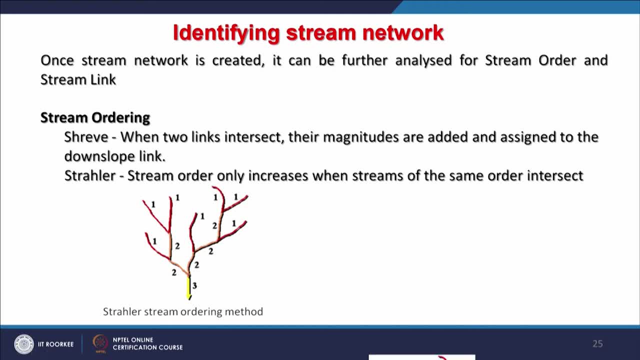 This is STELR scheme of ordering, stream ordering. Now, if we go for this, first the SHRIB, when two links intersect, their magnitudes are added and assigned to the down slope link. it is a kind of addition Example here for the same schematic drainage network that first order, first order meets. 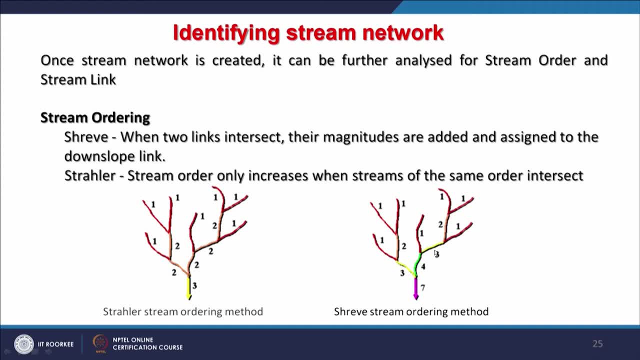 it becomes second order. When second order and first order meet, it becomes third order in the down slope side. When this happens, first order and third order meets, it becomes fourth order. When third order and fourth order meet, it becomes seventh order. 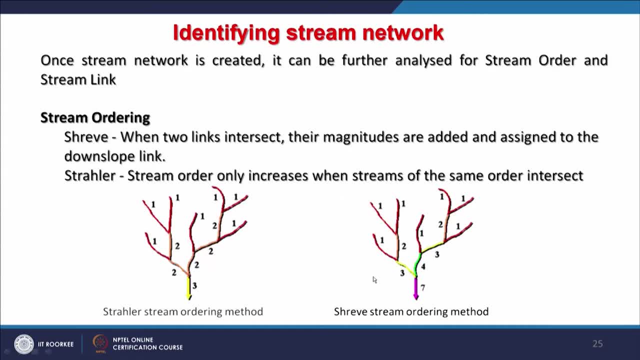 So in SHRIB, ordering what we are seeing, that at the outlet we are having a seventh order, whereas in case of STELR it is just third order. So this is the third order. So this is the third order. 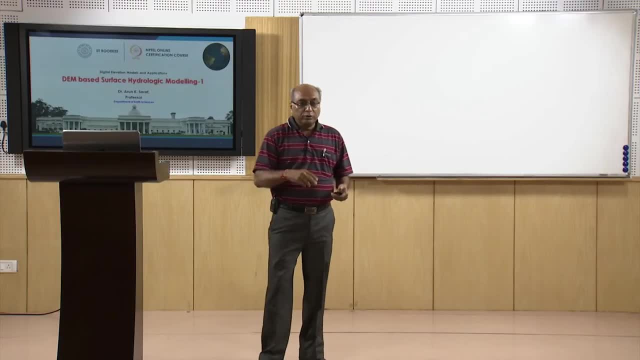 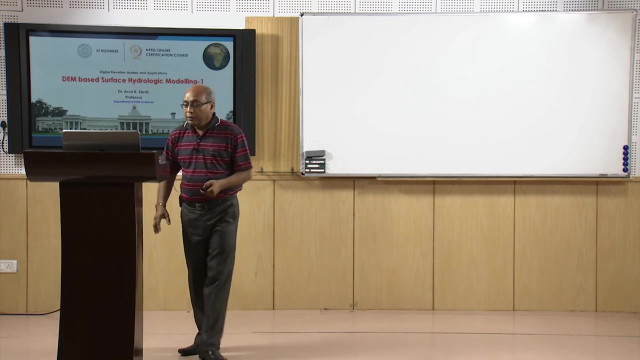 So this is the third order, Though the drainage network is same because of two different way of ordering streams are there, So both options generally have been implemented in popular GIS softwares. Depending on our requirement, we can choose, but this one becomes more SHRIB, one becomes 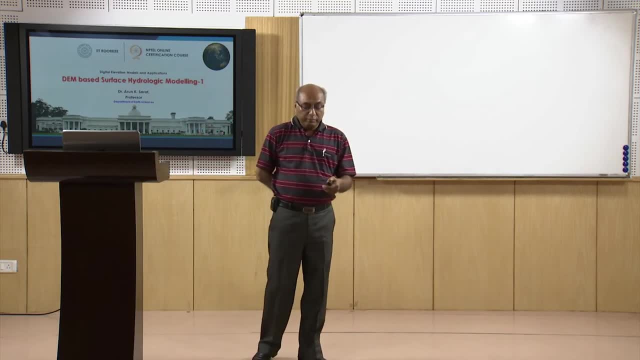 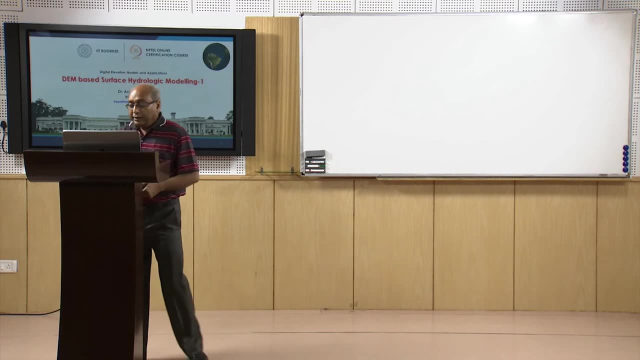 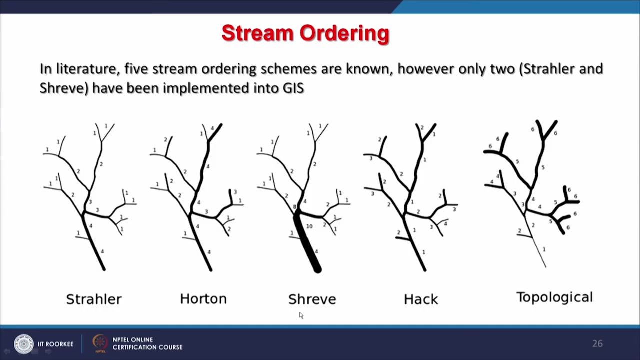 very easily understandable and it is therefore very much popular. Now there are other stream ordering schemes are available in literature. Some of them have also been implemented on GIS. So five popular one are shown here. Two: we have already seen STELR and stream ordering. 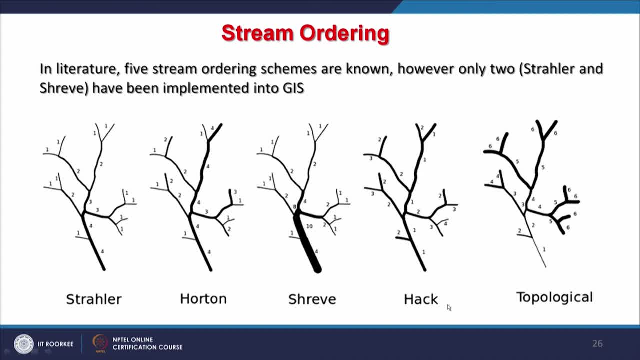 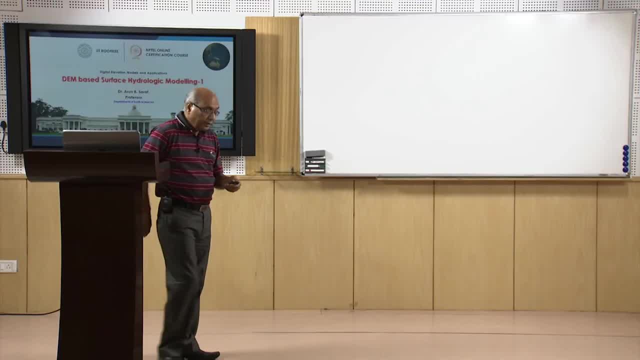 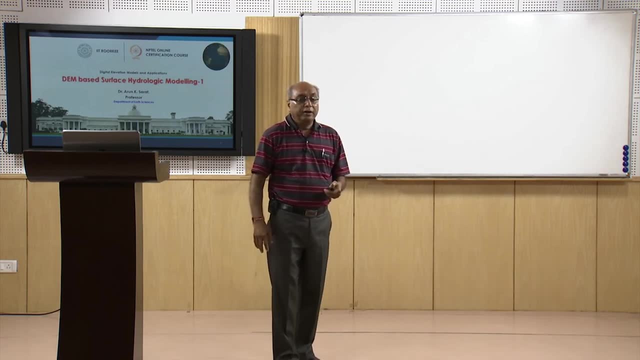 Then there is a Horton stream ordering scheme, There is a HECK stream ordering scheme and there is a topological stream ordering scheme. Different schemes are there. So these are the three. One can follow any one, or the most popular one, which is the SHRIB one. 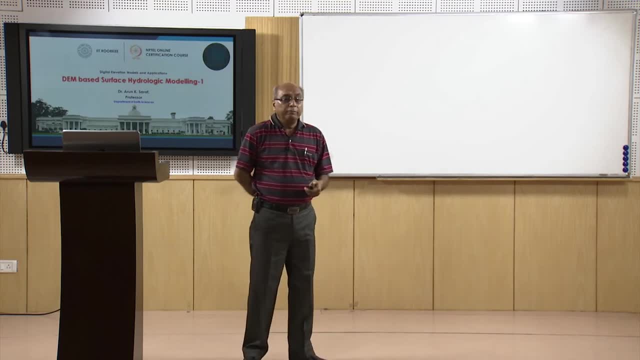 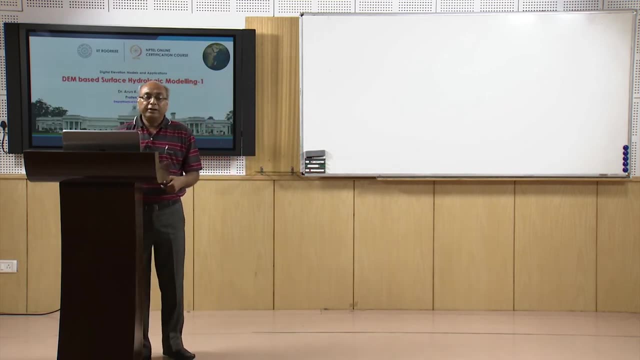 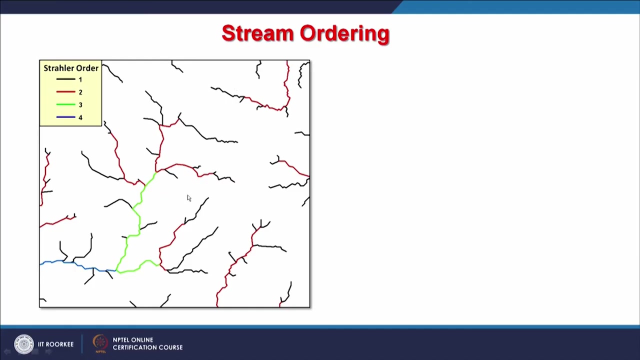 And these are the two which are most popular Now, if I take our example digital elevation model, on which we have generated our this flow direction, and then later flow accumulation, and then stream network, Once we put this stream network for this STELR, Then this is what the output we get for our example digital elevation model. 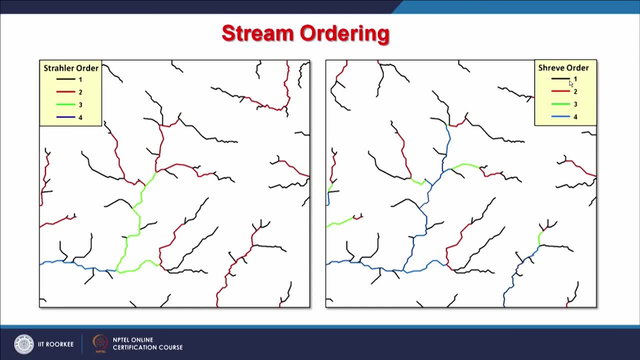 And if it is subjected for a SHRIB order, then this is how it looks, Though the drainage network- overall drainage network- is the same, But when we apply two different stream ordering schemes then we get slightly different results here. So, depending on your requirements, one can choose any one of these ordering schemes. 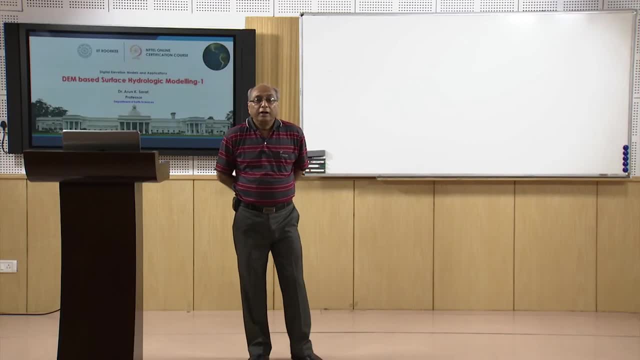 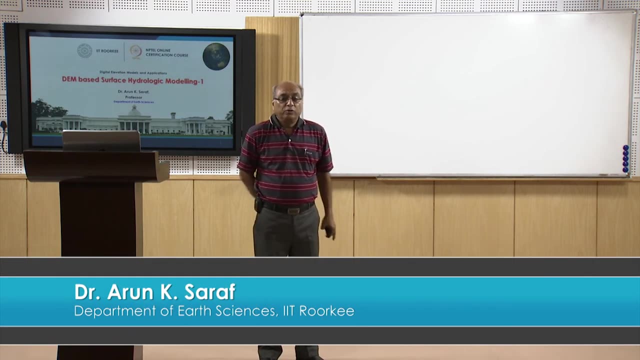 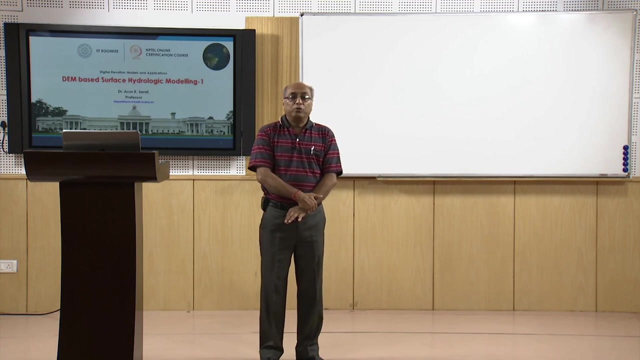 Thank you. So this brings to the end of this discussion. This is: this is in the surface hydrologic modeling is in two parts: The first part we have discussed. in next lecture we will be discussing the second part of surface hydrologic modeling.